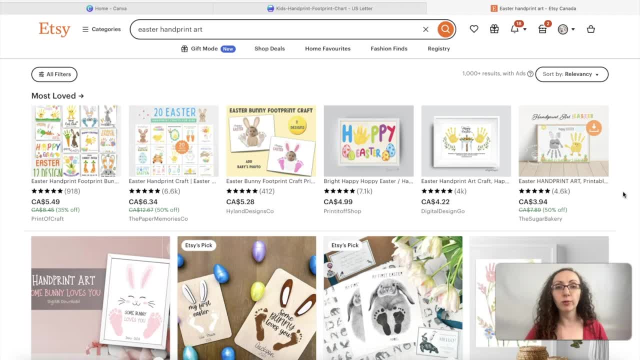 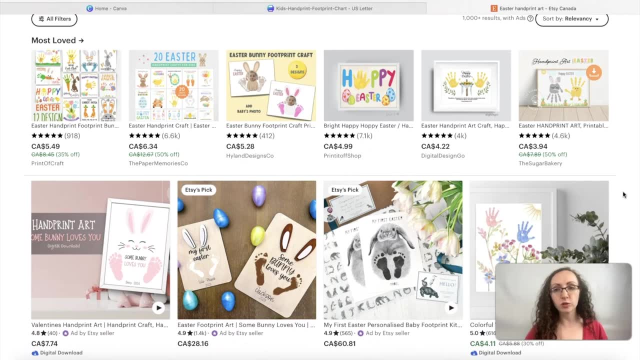 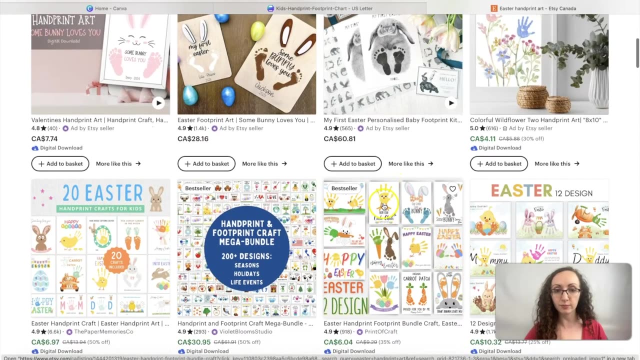 have been used for in other designs, but we are going to be creating our own unique design based on that inspiration. so handprints are often used to replace either an element in the design. so, for instance, here we have: the handprint becomes a chick, the footprints become bunny footprints. 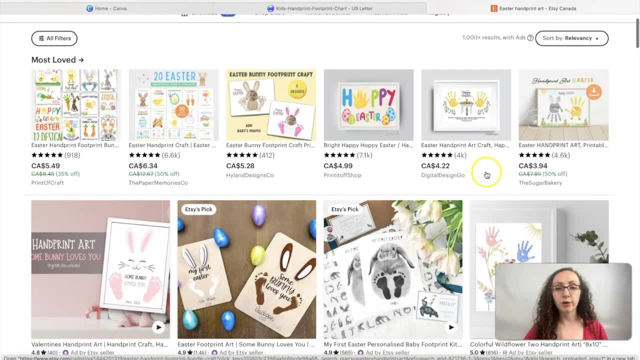 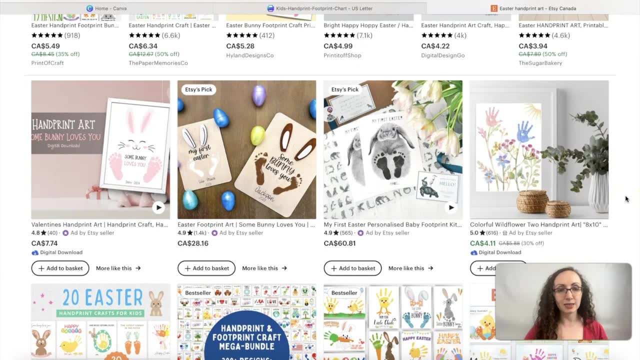 they can become carrots, like we see here. the handprint can be used to replace a letter in a word like happy easter. so we're just looking to get an idea of what other sellers have created. but we are going to be creating our own unique design and not copying someone else's. 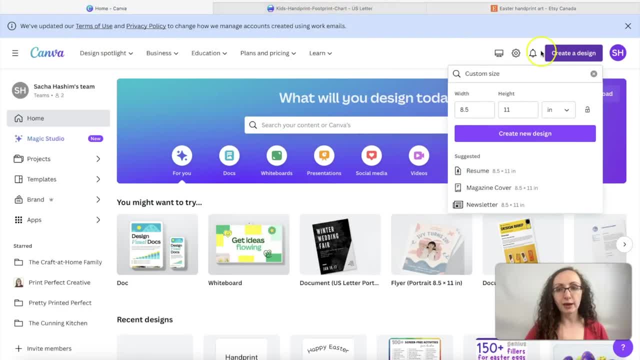 once we have found some inspiration, we're going to go into canva, click this, create a design button and then choose a size. so i've typed in 8.5 by 11 inches, because that is the most standard paper size in north america. you're going to want to make sure that you have the right size for your design. you're going to want to make sure that you have the right size for your design. you're going to want to make sure that you have the right size for your design. you're going to want to make sure that you have the right size for the US letter. 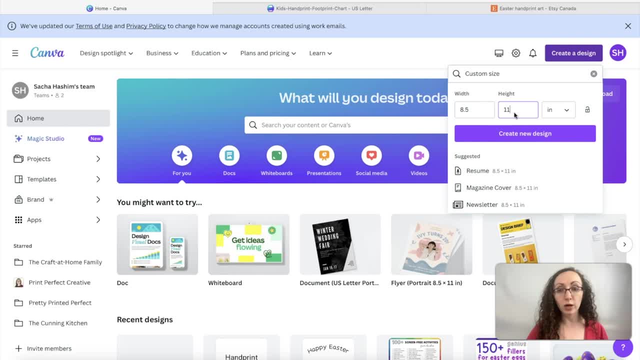 if a lot of your customers are based in Europe, you may want to adjust this and make it a four size, which is international standard, but for me, my biggest audience space is in north america, in the united states, so i'm going to be making it 8.5. 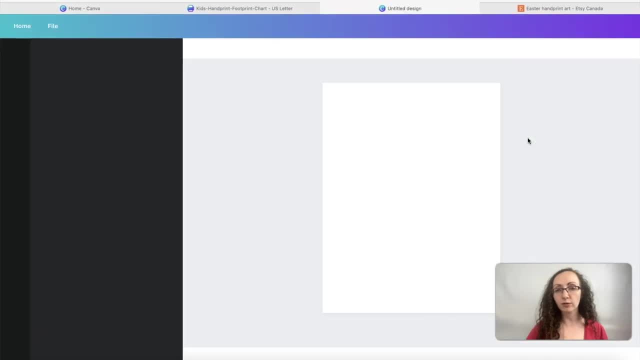 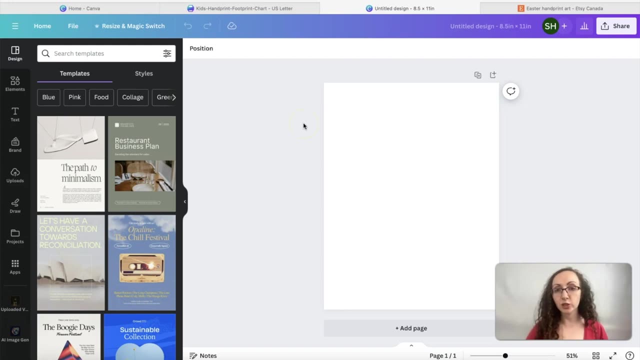 by 11 inches. so i'm going to create new design right here and one thing i will specify for the size is 8.5 by 11 is a standard size for printing, but it is not really a standard size for picture frames and your customers are probably going to be wanting to frame. 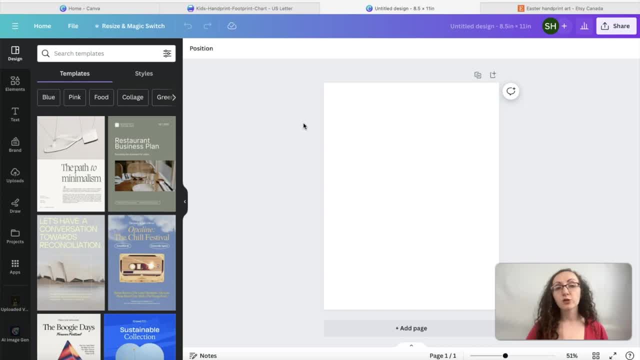 the artwork after they've added their child's handprints. So if you want to make it as user-friendly as possible, what I would recommend is leaving some white space all around, and what that will allow is that your customers can print out the template on US letter-sized paper- 8.5 by 11 inches. but 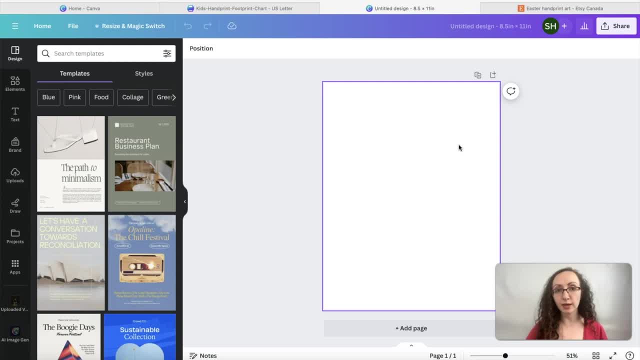 then they can actually cut out some of the blank space that's on the outside and they'll be able to fit the finished artwork inside an 8 by 10 frame, which is a standard size for a frame. That way, you have the best of both worlds: your. 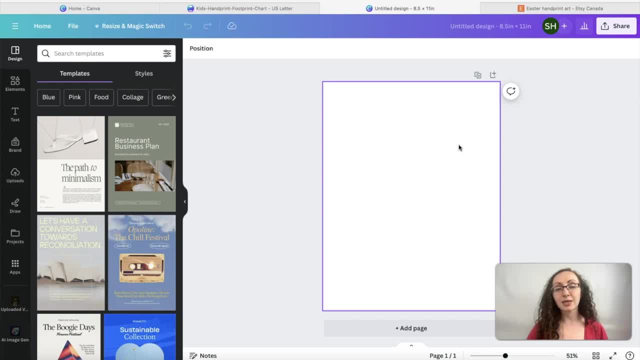 printable will be easy to print for your customers, but they can also easily fit it into a standard sized frame. So the first thing I want to talk about is how you can print out the template on US letter-sized paper. So the first thing I want to talk about is how you can print out the template on US letter-sized paper. 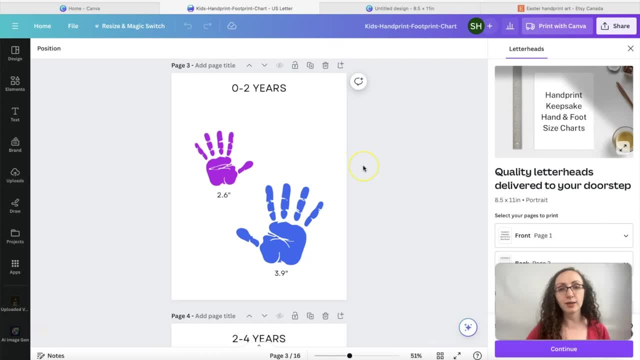 The first thing I'm going to show you is the size chart that I created, that I'm going to link below so that you can use it to help you create your handprint art. What it is is: I created a chart that shows standard hand sizes, average hand. 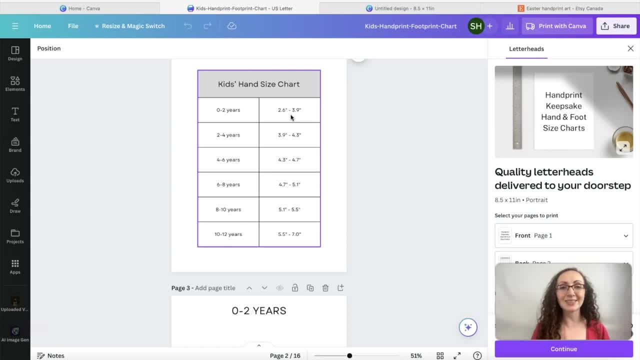 sizes. so I mean, not every child is going to have the exact same size hand or foot, but this is just to give you a rough idea of what to expect in terms of hand size for different ages. I made it go from 0 to 12 years And just to show you so this would be the hand size that a 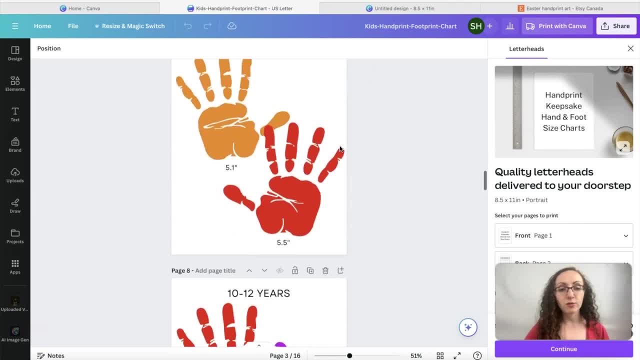 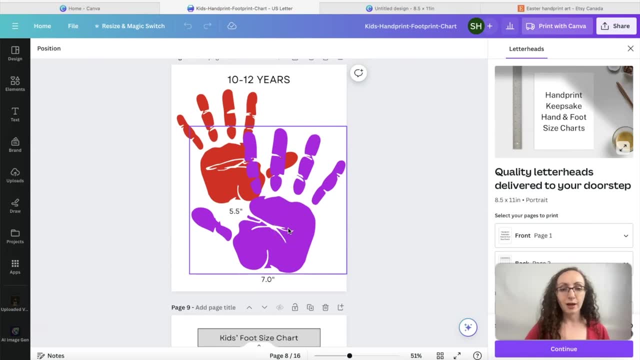 newborn would have on average and if we go, keep going, you'll see the hands keep getting bigger. this would be the hand size of the average 12 year old. Customers may not be making this hand print art with a 12 year old, but I 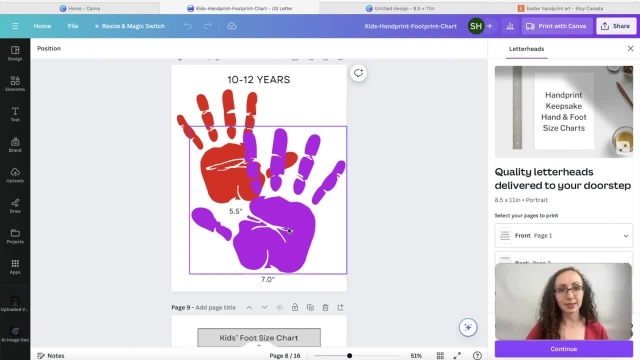 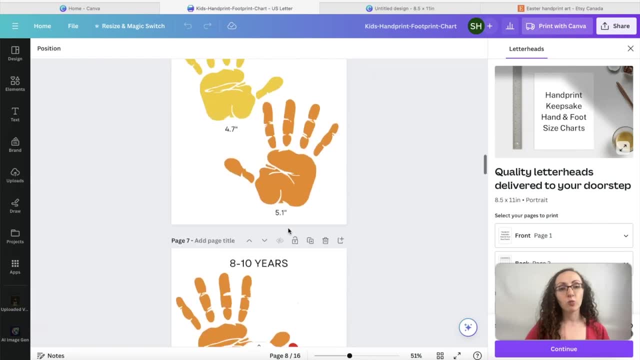 wanted to include them all, just so that you have a realistic idea of what to expect. What you will want to do is make sure that your hand print art template works at least up to the ages of four or six years old, unless it's something that's really specifically meant for babies or 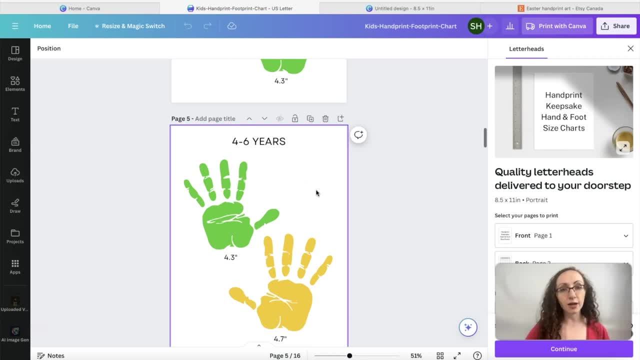 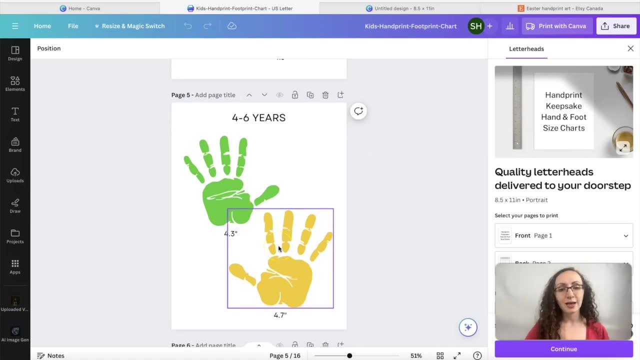 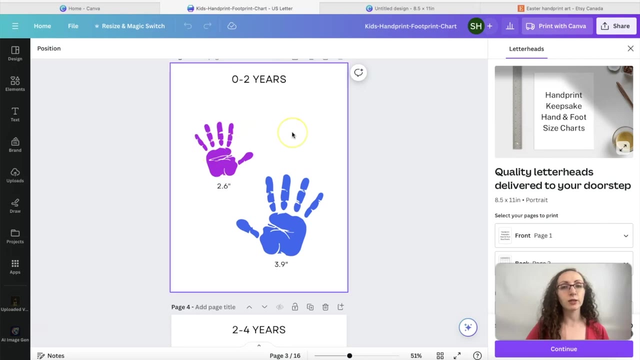 newborns, which may be the case, But if it's not, make sure that your customers can use it at least up until four or six years old, because if the only way that your design works is if the hand is this size, then it's not going to be totally. 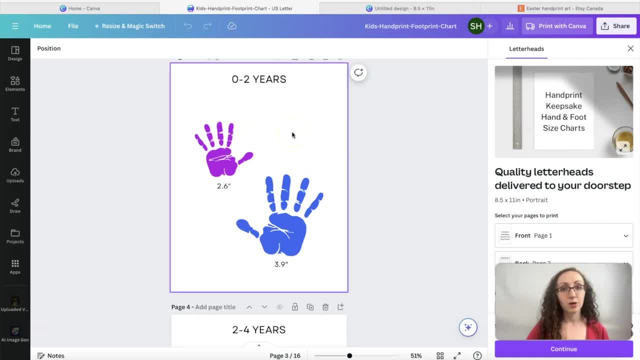 useful for your customers, because some people may want to make it with children who are three, four, five, six years old, So that's something to keep in mind when you're creating hand print art and footprint art. I've also included the. 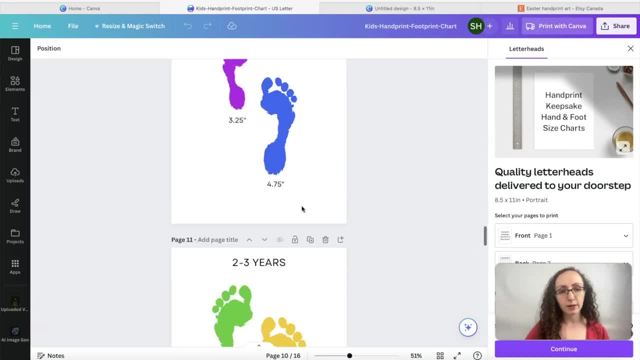 footprints. if you keep scrolling, so this gives you an idea. So like this would be 0 to 1 year, 4 to 5 years, so just try to keep that in mind when you're creating your designs. So we're going to go into here. 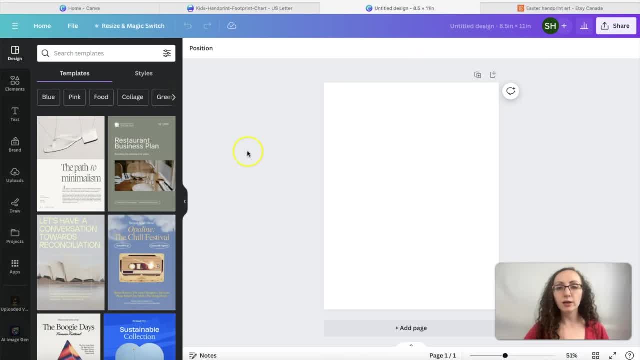 and start creating our design. We saw a lot of cute little templates where the hand print became a chick, So you can add graphics to your Canva design. You can either get graphics from a site like Creative Fabrica if you have a subscription, or you can go find elements right here in Canva. So we're going to 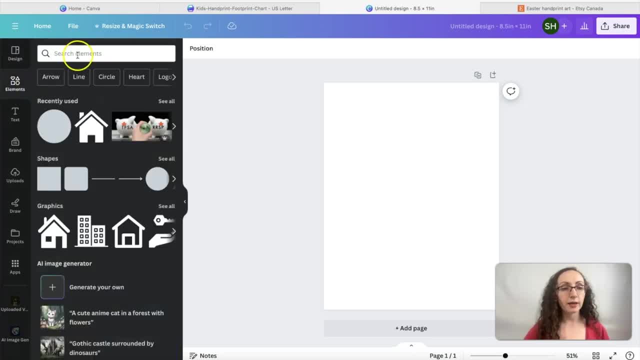 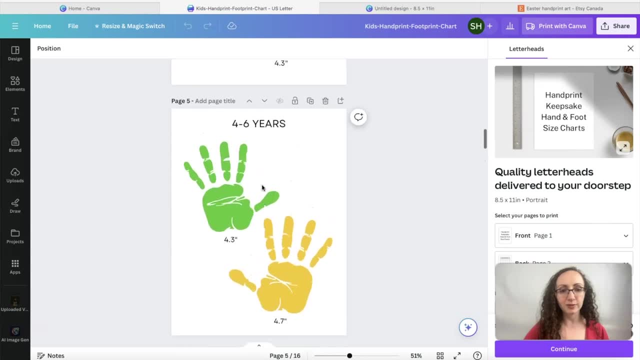 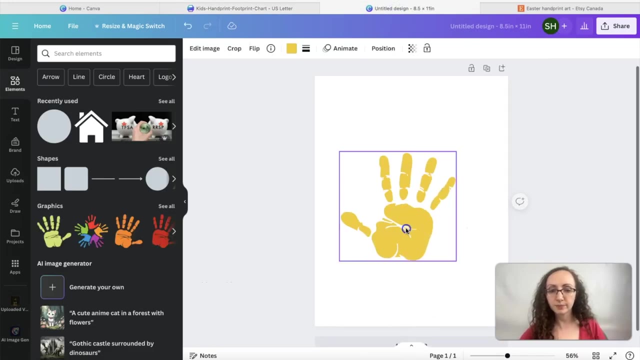 click elements here on the left, the left, And I'm going to start actually by adding a handprint. So I'm going to take a handprint, maybe of a six year old, Go add it here, copy and paste, And I'm going to put it in the 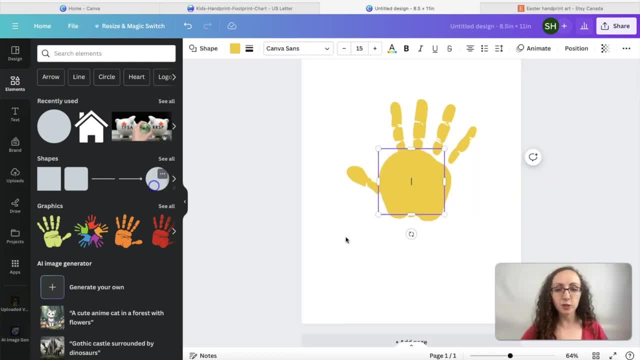 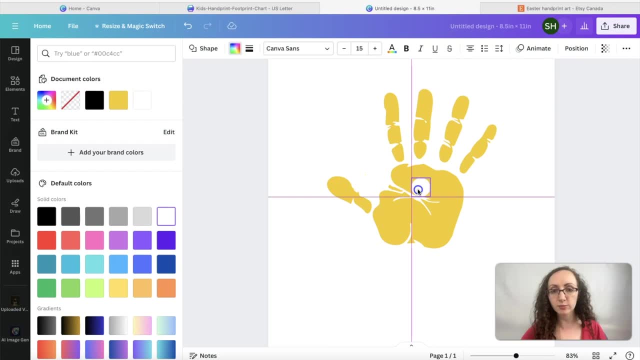 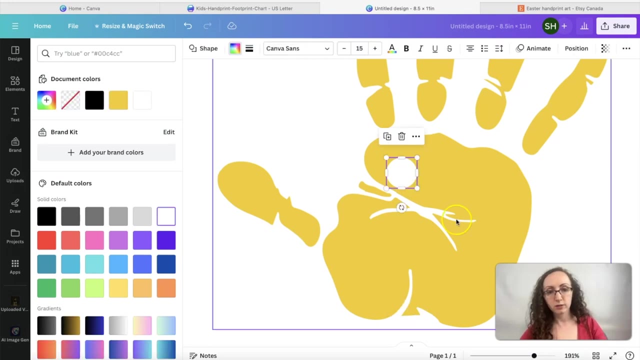 middle, and this is going to become our chick. If it's going to become a chick, I should probably create some eyes for it. Now, the eyes are something that your customers are going to have to add after they add their child's handprint, So I'm just making eyes out of little circles. 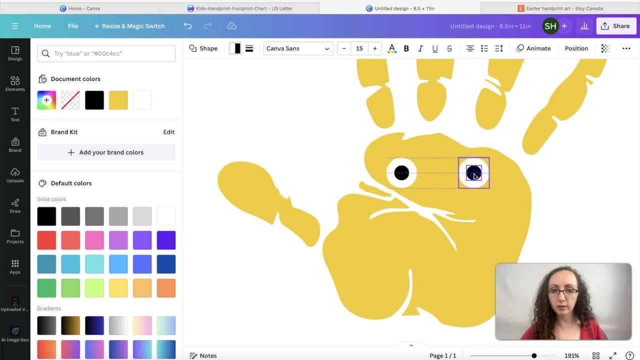 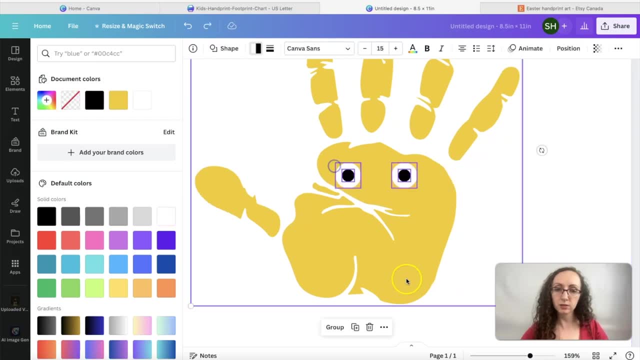 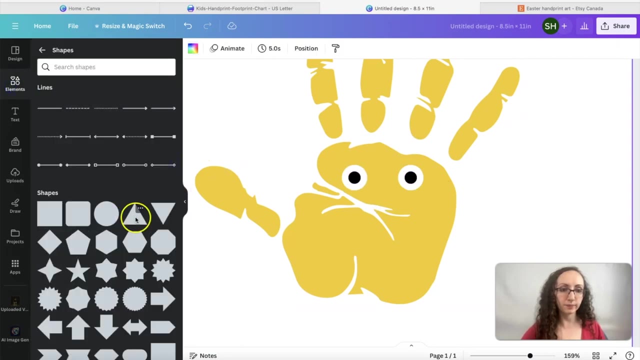 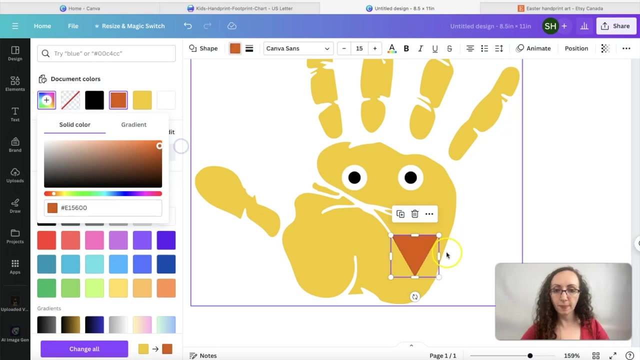 Do it like this: create another eye, add it here- Maybe we can center it a little bit That- and then they're going to need a beak. So if I add an orange beak, choose the color right here. All right, so it'll look something like this once you're custom. 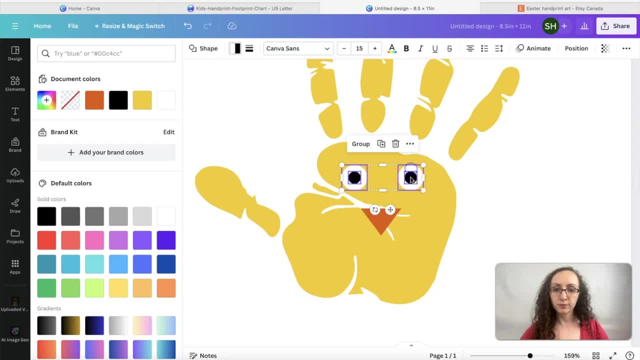 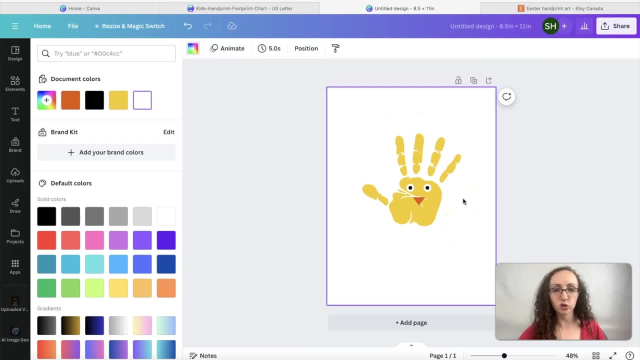 Now, like I mentioned, these are elements that your customer is going to have to add after they add their child's handprint. In general, you're going to want to avoid having your customers add things to the design or, at the very least, make the things that they need to add. 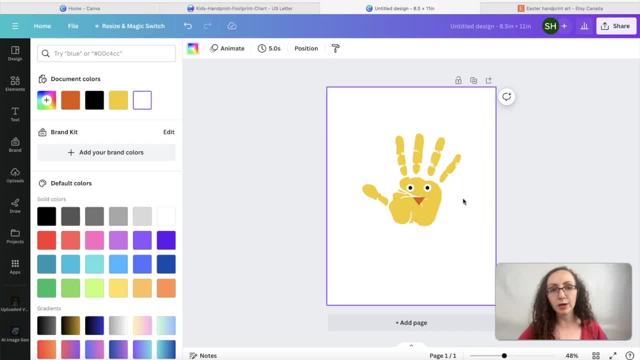 as simple as you possibly can, Because the point of these handprint art templates is that your customers can just have an easy craft to create a keepsake from their child's handprints. So they're just going to want to print them out, add their child's handprint and be done with it. So you 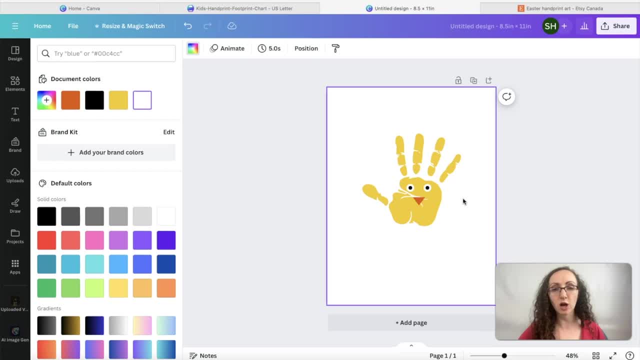 want to avoid having graphic elements that are supposed to be on top of the handprints or footprints, because the handprints or footprints are the things that are going to go on last, after your customers print it. So if we wanted to add, for instance, some grass, 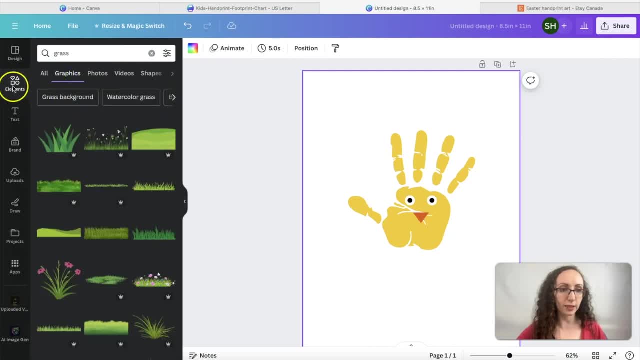 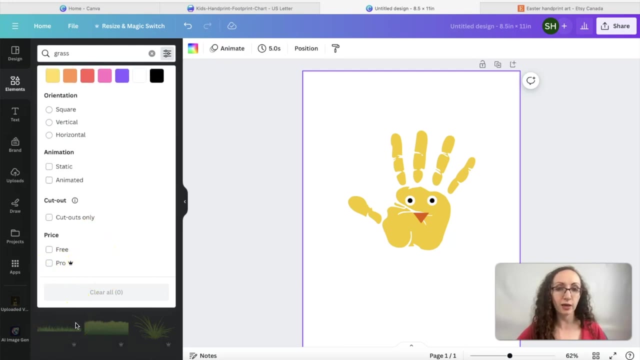 go under graphics So we click elements in Canva. We went and typed grass at the top At the time of this recording. in this sort of template you would actually be allowed to use pro elements if you have a Canva pro account. The licensing currently for Canva, but I encourage you. 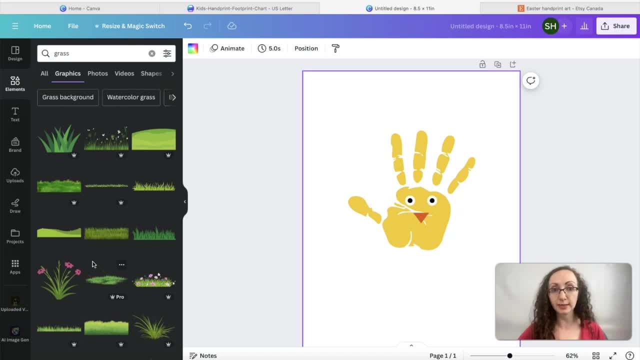 to double check this before you use any of Canva's elements in your designs. But the licensing currently is a bit different. So if you have a Canva pro account, you would actually be allowed to. currently allows for you to use ProElements in designs that you are going to sell, as long as 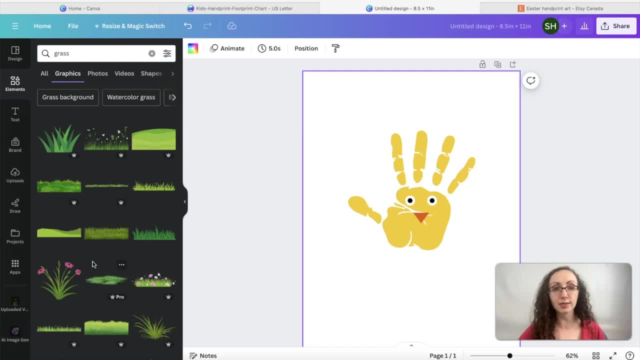 they are designs that will not be further modified by your customer electronically after they purchase it. So in the case of handprint art, they're not going to be editing the file any further after they download it. They're simply going to be printing it out. So the licensing right now would 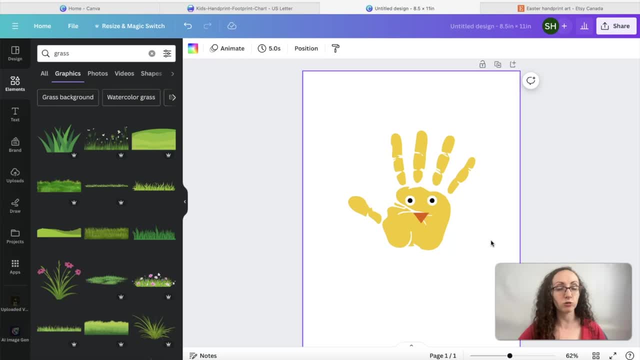 allow you to use ProElements in your design, but I encourage you to double check this before you use anything in your designs. This is not legal advice and I don't want you to get in trouble for it, So make sure that you're always clear on the licensing for what you're using And if you're 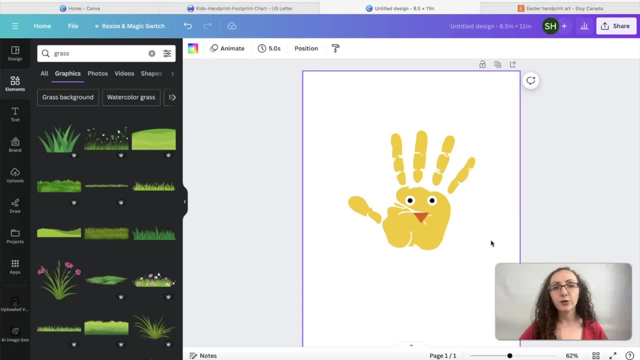 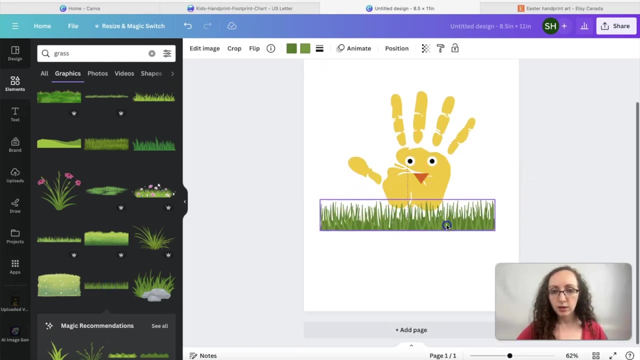 not sure for Canva, or if you can't find what you need in Canva, you can go get external graphics from a site like Creative Fabrica. So if I add grass here, maybe we can add. let's see, what does this one look like? This one's cute. So what I was trying to show you. 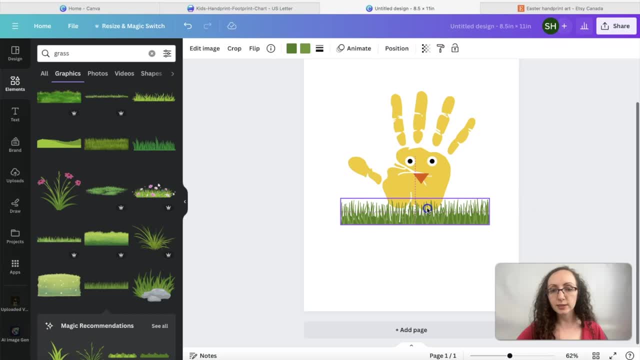 before this all started was that you don't want to have designs like this, where the grass is supposed to be in front of the handprint, because when your customer's at the handprint, it's going to be on top of everything. So if there are little details for them to add, like eyes or a beak on. 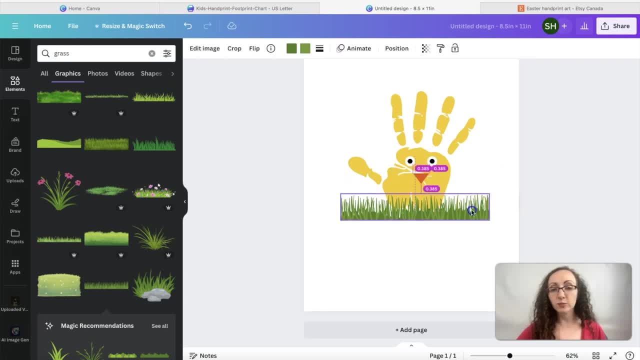 this chick. that's fine, But trying to put this grass in front of the handprint would be a huge pain for your customers, because they would actually have to print out two copies, cut out the grass and then glue it on top of the. 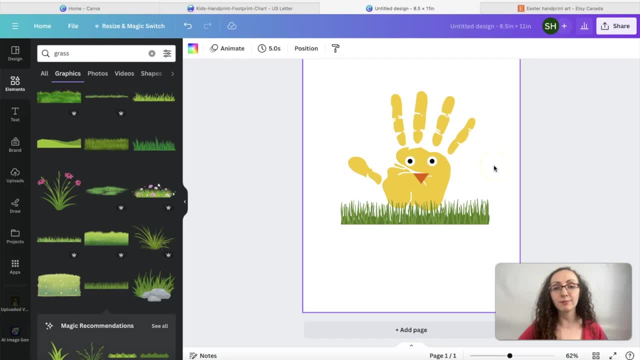 handprint. So be mindful of that when you're creating your designs and make sure that the only things that are supposed to be on top of the handprints or footprints are things that your customers can easily add, like these eyes and this beak. So we added grass. We can maybe tweak the 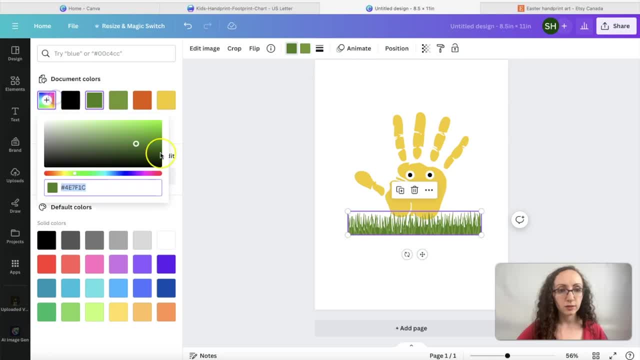 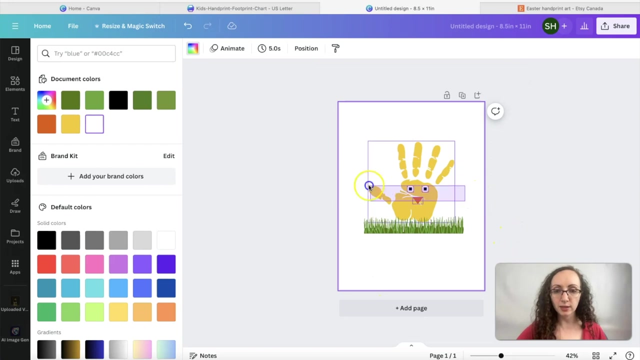 colors a little bit. Some of the elements in Canva are color changeable, So this was one of them, So I'm going to change that color and then the lighter color, making it something a little lighter like this: Perfect, All right. So we've added some grass, though we are going to make sure that this is the front like. 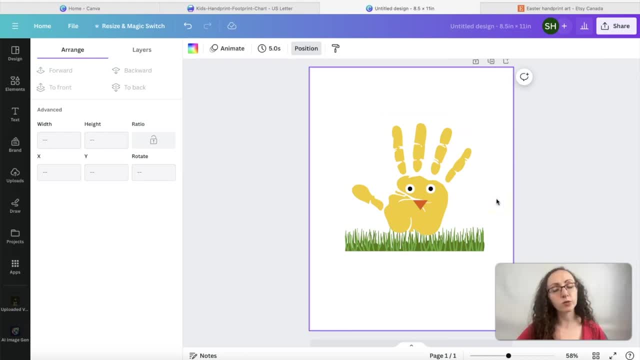 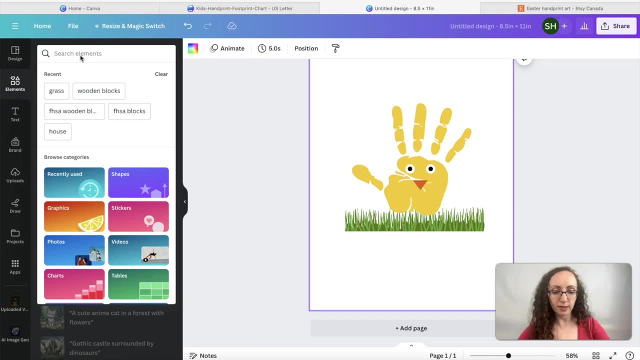 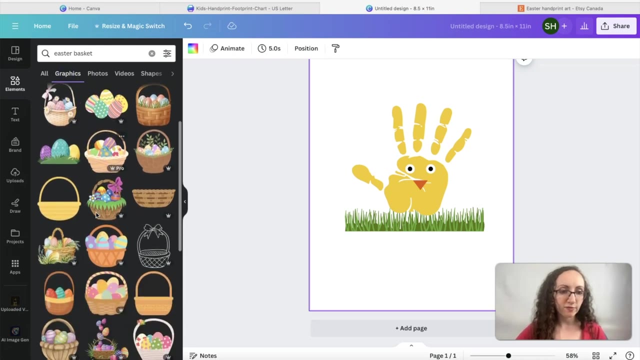 this. We're going to want to add some grass to the front of the handprint, So we're going to add some more graphic elements here, So we could add, for instance, an Easter basket. So if I type in Easter basket in Canva, go under graphics and then find something that I like. 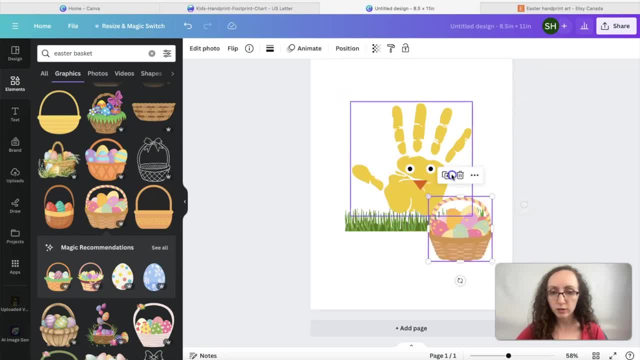 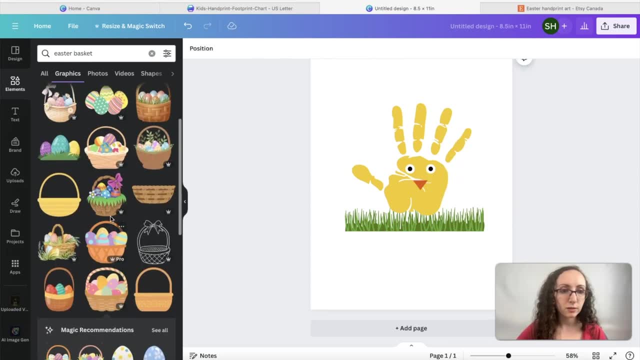 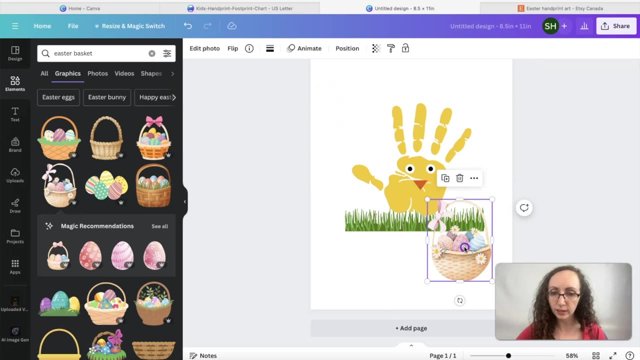 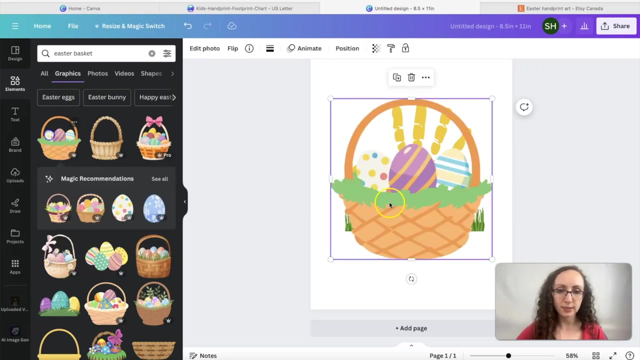 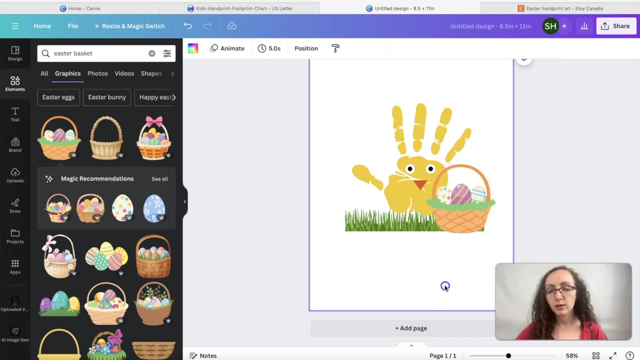 This is kind of cute. Could that work? Maybe not. Let's choose one that we really like. This one's pretty cute. It has this water color effect going, Or just this basic one here, So you would choose one that you like. You can add it here. We're going to have to move our chick. 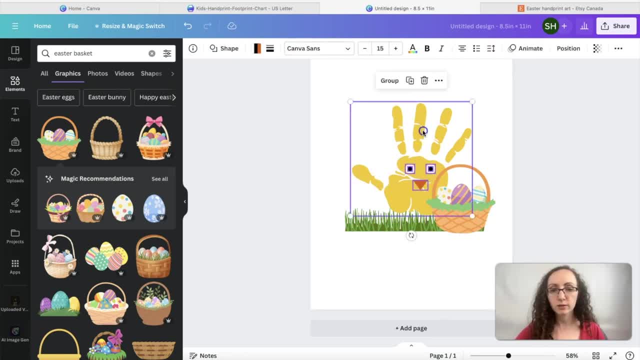 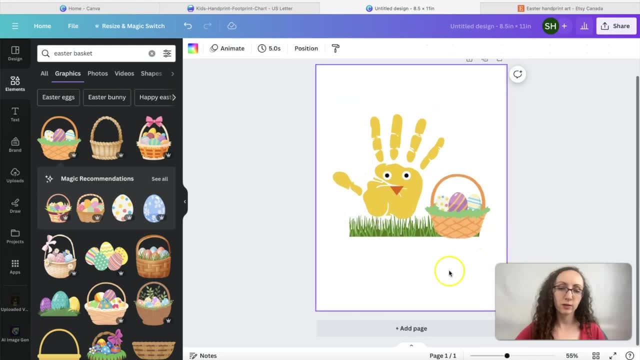 but that's okay. So if we move our chick here, that's fine, And here we're layering the elements, which is going to help you comply with the terms, to use the graphics. You're always supposed to layer the graphics, modify them in some way. I could. 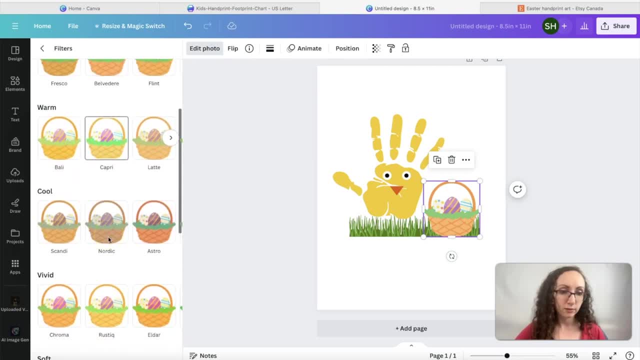 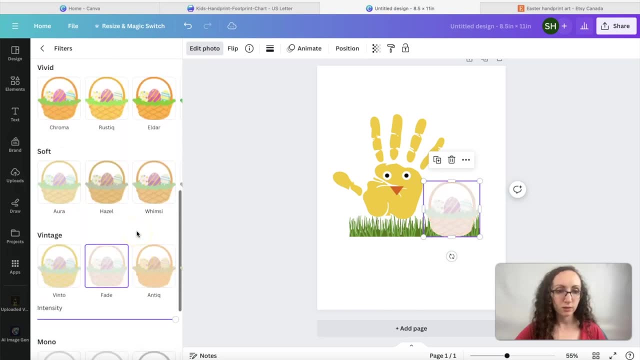 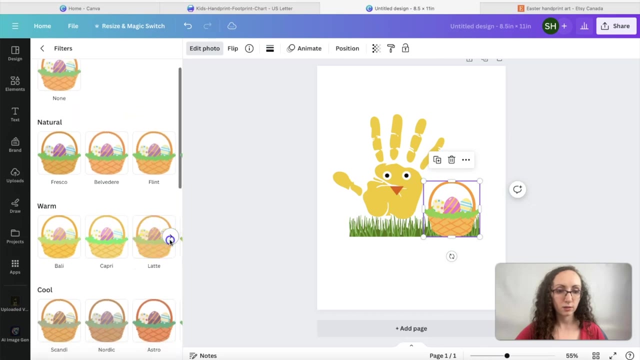 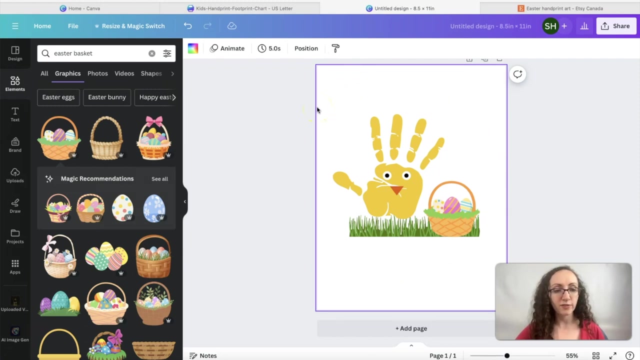 for instance, go modify the colors here. Maybe not that effect, Maybe something like this. The reason you're going to want to modify it is, like I said, to comply with the licensing terms. Graphics need to be modified or layered. Basically, you don't want your customers to be able to extract the graphics in any way. 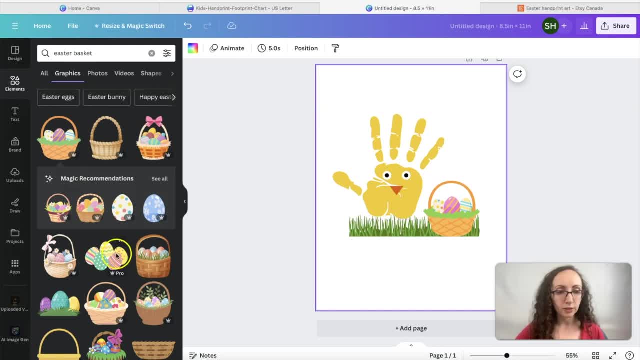 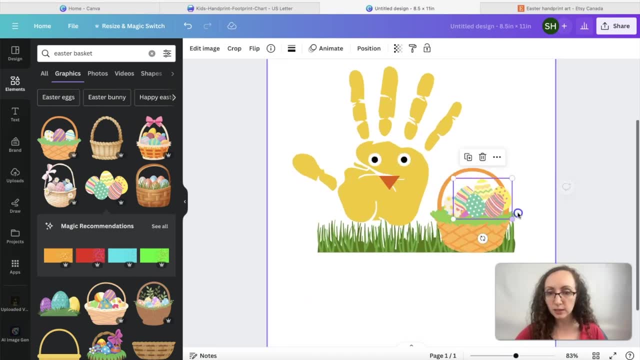 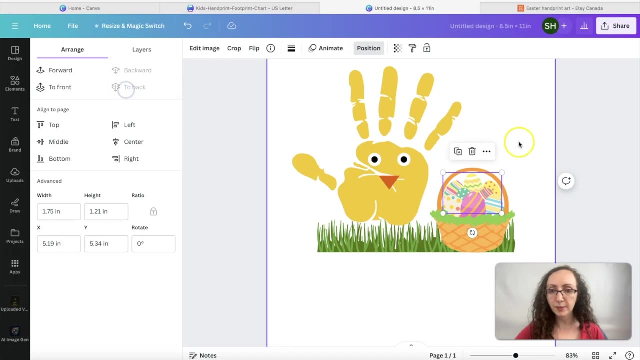 and then use them for other projects. So we can also maybe add some more Easter eggs. So we could add them. They could be actually in this basket, So you could go and click this position button, send them to the back. and now there are more. 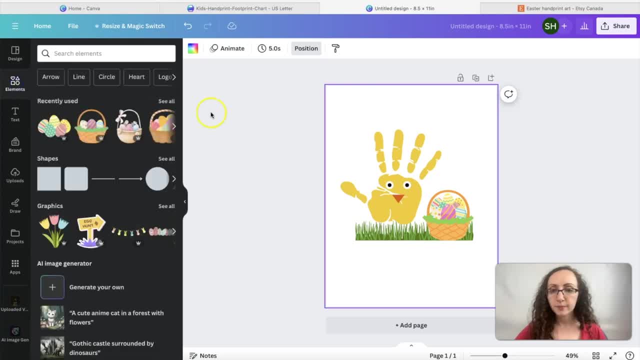 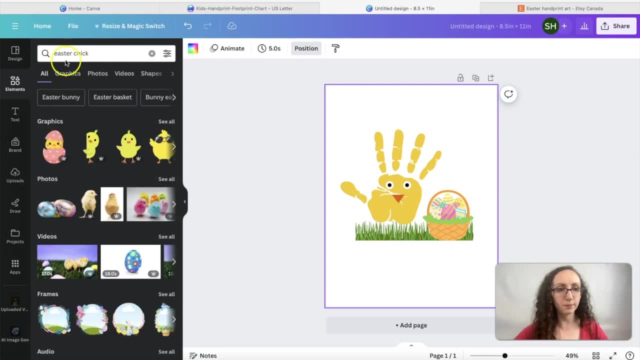 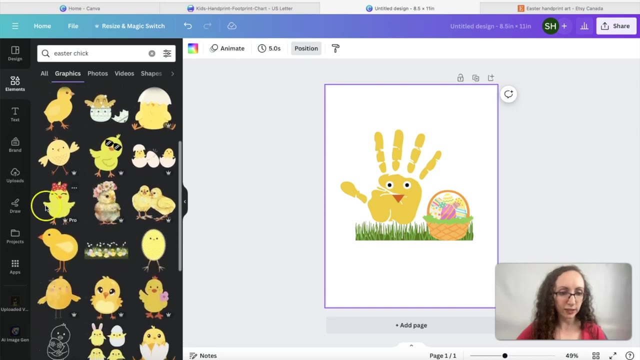 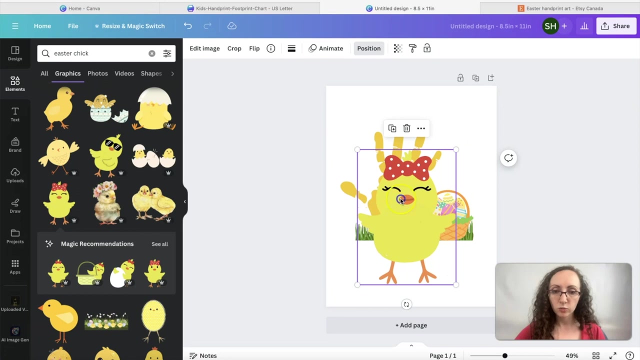 eggs inside your basket. We're going to also want to add legs for your chick. So if I type in Easter chick, look under graphics and then I'm going to find an Easter chick that has little feet that we can use. So we could use this one. 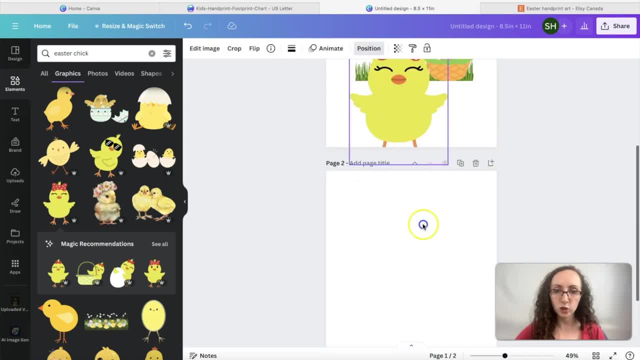 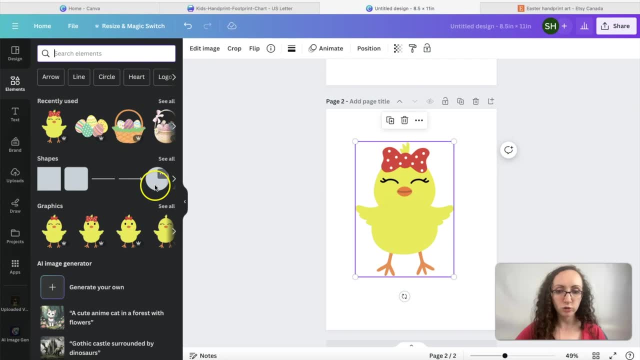 So what we would do to use it. I'm just going to temporarily add a page so that I can show you what we need to do. So we added the chick. We're going to go choose some shapes like this. It can be a square. 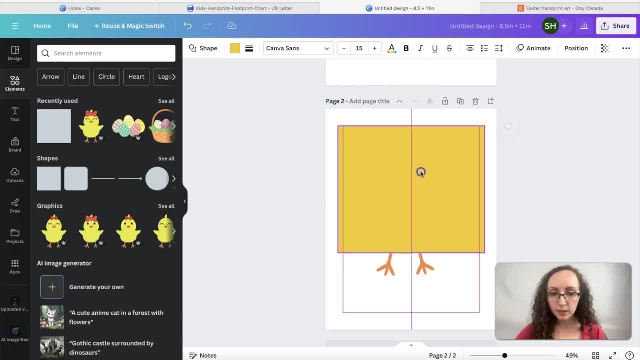 It can be a circle. It depends on the shape that you're trying to hide. And then, if we drag it down to hide the body of the chick, We're going to make this white. There you go. That leaves us here. We can see a tiny little bit of the chick, and now we can. 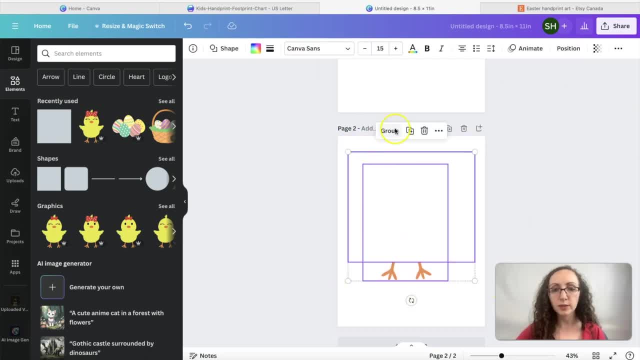 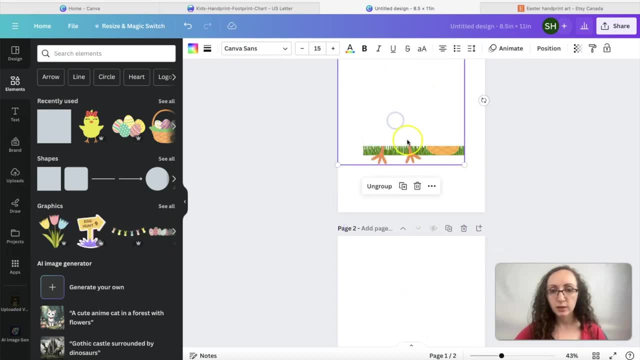 And then I can select both of them by dragging a box over them, Click group, And now, when we move them, everything moves together and the chick continues to be hidden. Now, what I'm going to do is I'm going to bring that into this design. 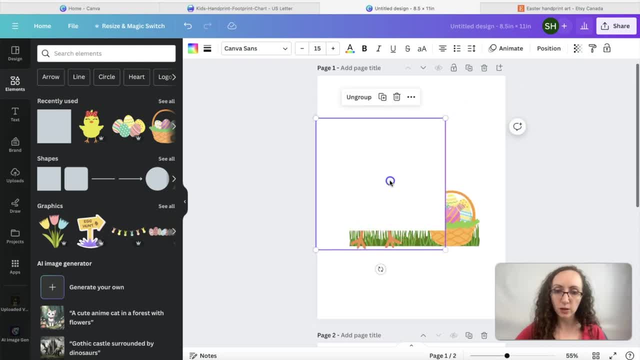 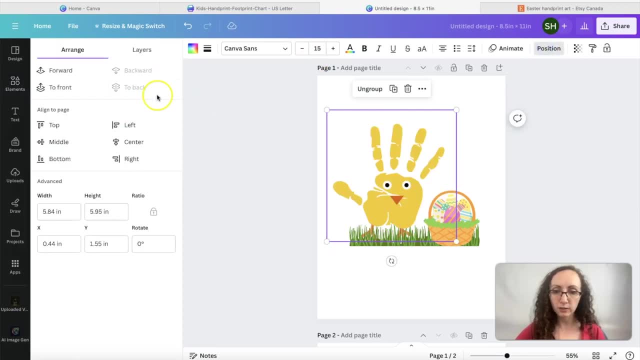 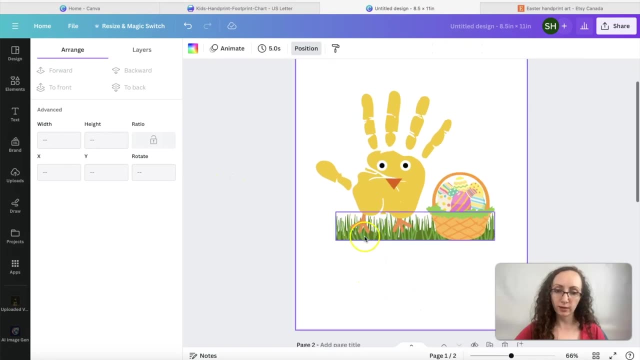 I might make it a little smaller, Just so that even smaller hand prints work, And then I'm going to send this to the back and maybe just a little bit forward. There you go. I sent it a little bit forward because that way the legs can be on top of the grass. 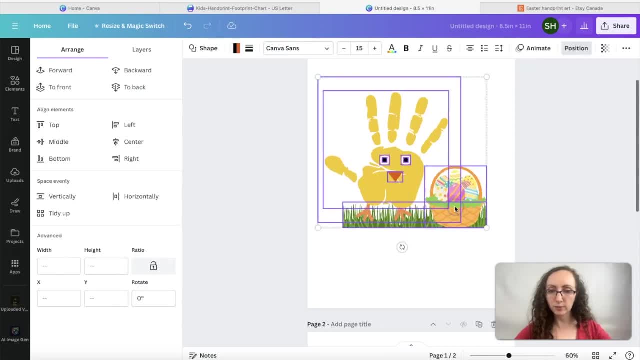 Now that is starting to look like something that could be used to create hand print art. So if I move- Whoops, Let's unselect this grass- I'm clicking shift so that I can unselect things while keeping the other things selected. 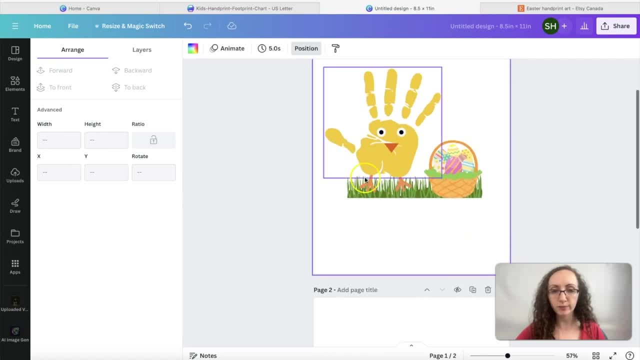 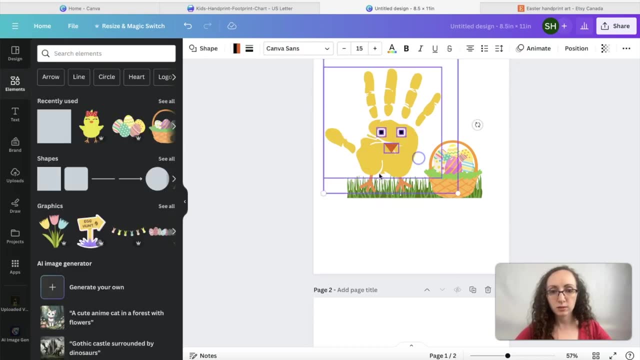 There you go. So now this design looks like this. That's pretty cute. Maybe move the hand print a little bit. There you go, So that there's, like I mentioned earlier, some white space so that your customers can frame this and put it in an eight by 10 frame. 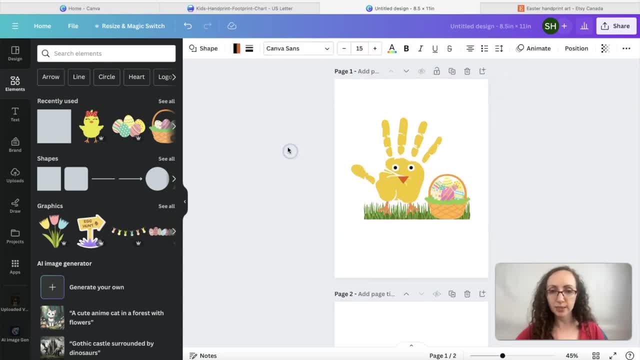 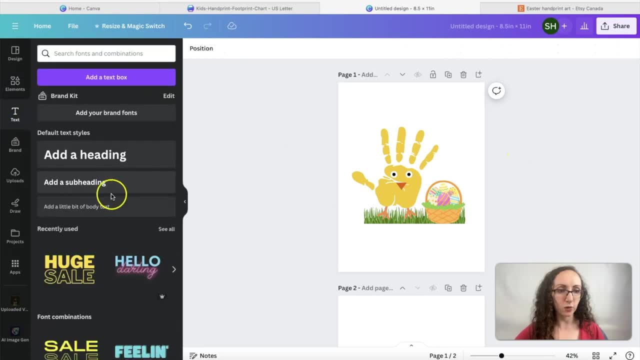 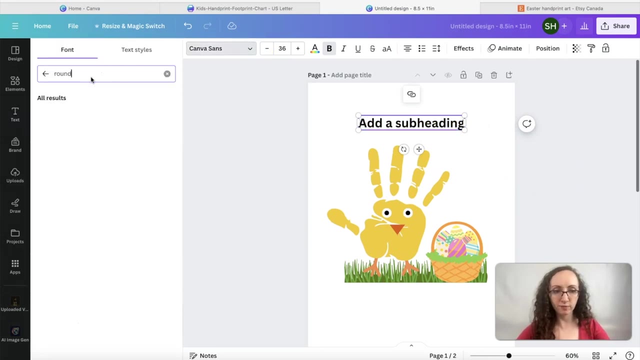 So the last thing we're going to want to do here is maybe add some text. So I'm just moving this and then we're going to go add some text. So I want it to say: Happy Easter. Let's go find maybe a rounded font. 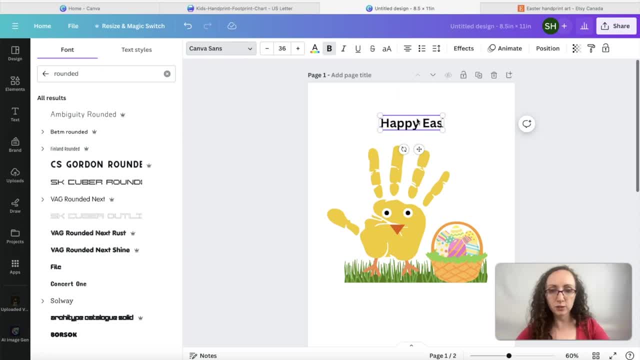 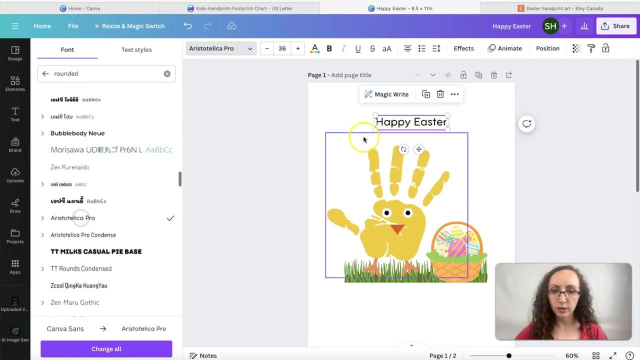 We can write: Happy Easter Whoops. Click on this and then go try to find something cute. There you go. Maybe not that, Let's see We're not going to spend too much time on this, but there you go, That's okay. 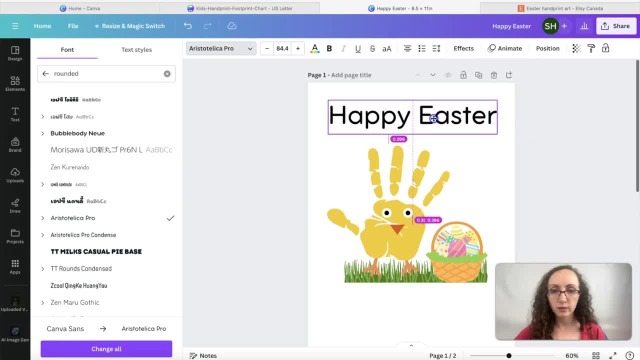 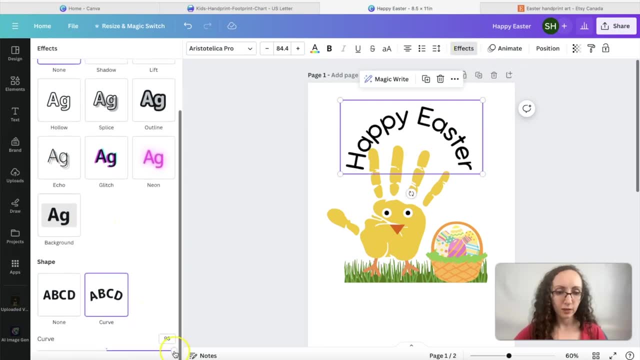 So if I make this bigger, and then I think this would look nice if it were rounded. So I'm going to go click effects curve and then maybe unround it a little bit, cause that's a little much. There you go. So it says Happy Easter. 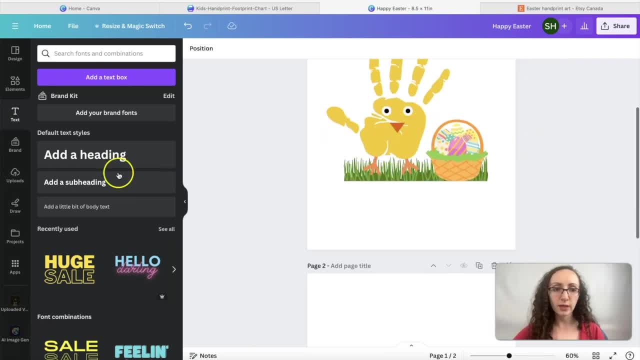 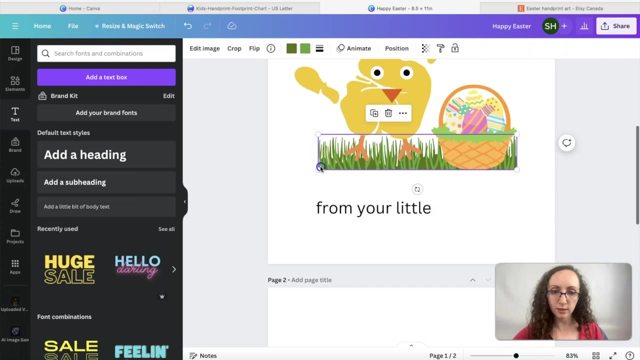 And then if we add just a little bit more text, we're going to say from your little chick, So we're going to increase the size here. I'm actually going to make this grass a little bigger. There we go. You do like this. 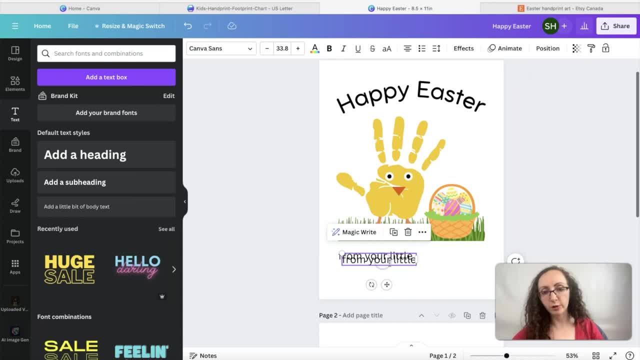 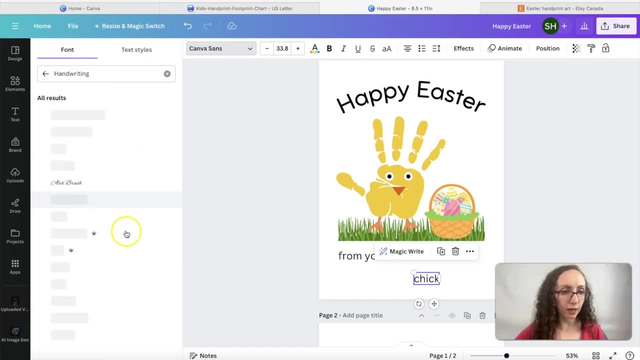 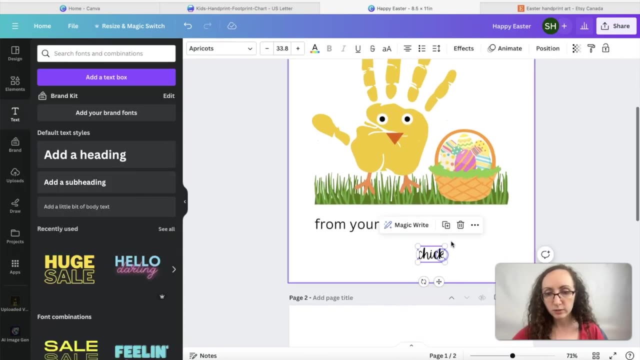 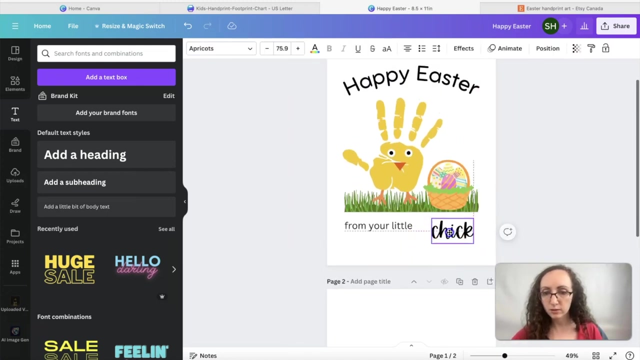 So from your little, and we're going to write chick. I'm going to make this font a little different. I'm going to go under handwriting and choose maybe apricots and look something like this: I'm going to make this a little bigger. 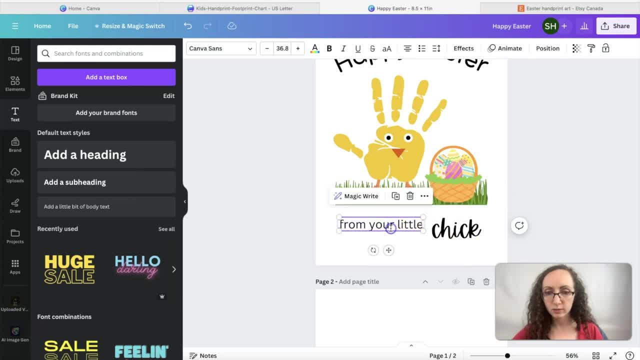 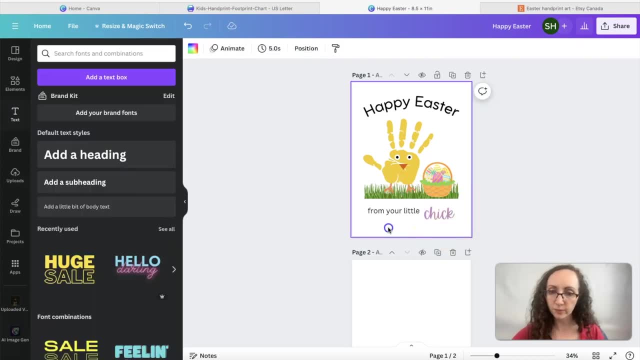 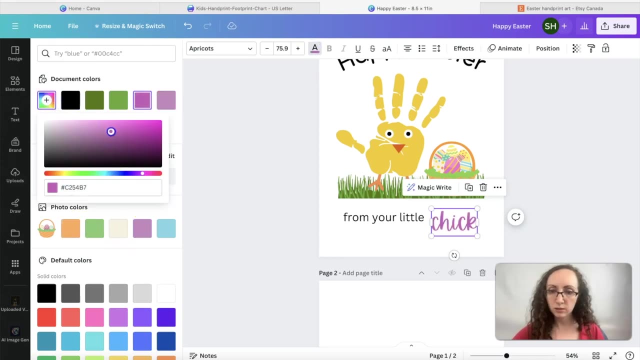 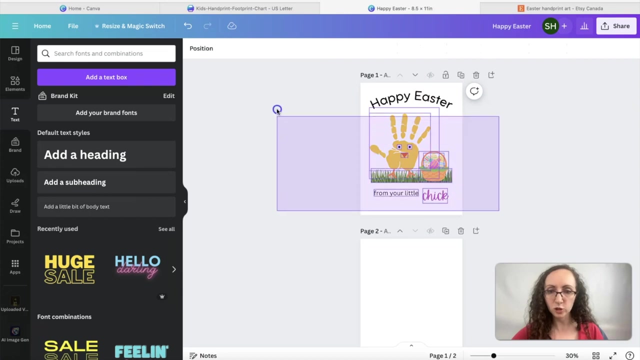 And then we can change the color. Maybe we can use one of the colors from this Easter basket. And there you go. So now this says Happy Easter from your little chick. I'm just going to bring it down a little bit, And there you go. 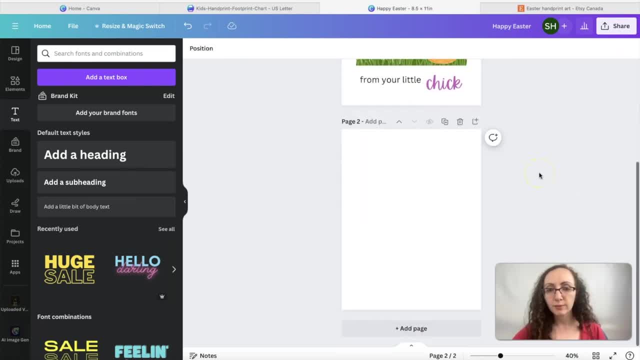 I think that's really cute. We can create a footprint art template as well, And then I'll show you how to package it for your customers. So there were several That had little bunny themed puns, So I'm going to make one here. 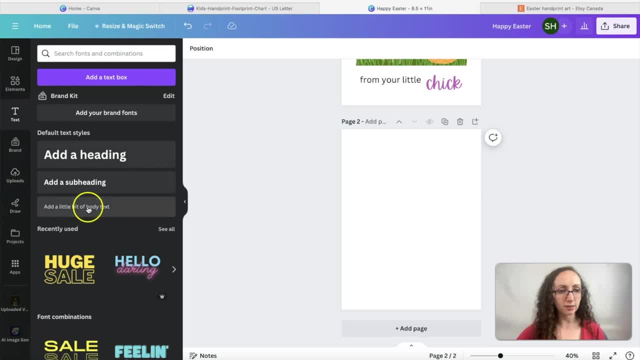 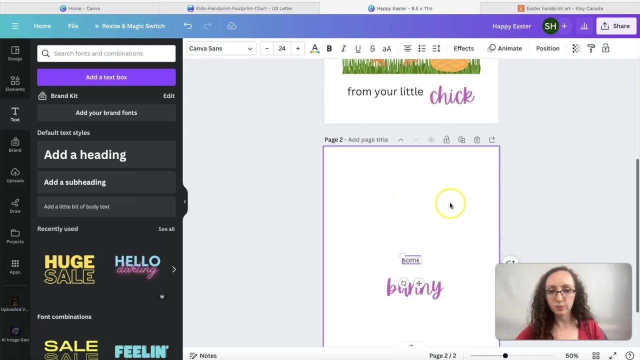 So we're going to want to add some text And we can have it say some: bunny loves you. So I'm going to take the same font that's here. I'm going to write: bunny, Make this bigger. Let's say: what was this size? 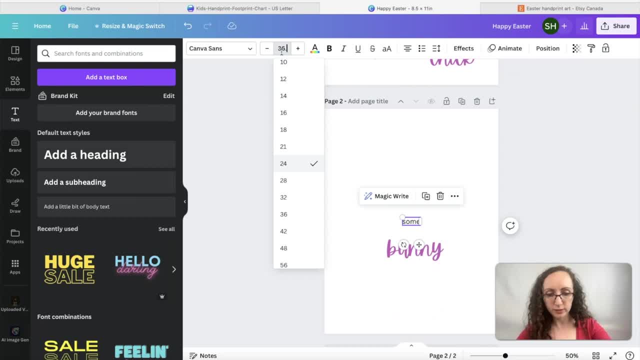 36.8.. Okay, 36.8.. Some bunny loves you- Whoops Loves you. Does it look better if it's on two lines? No, it does not. So some bunny loves you. We'll probably be changing the color after. 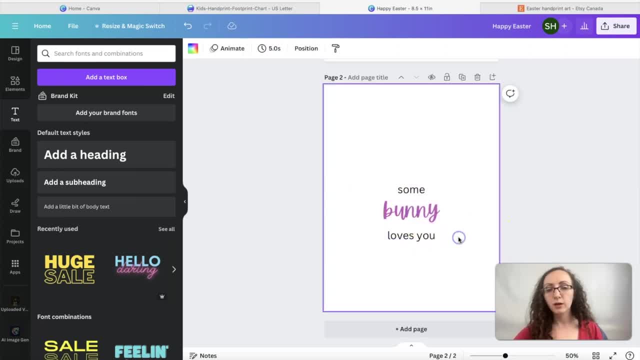 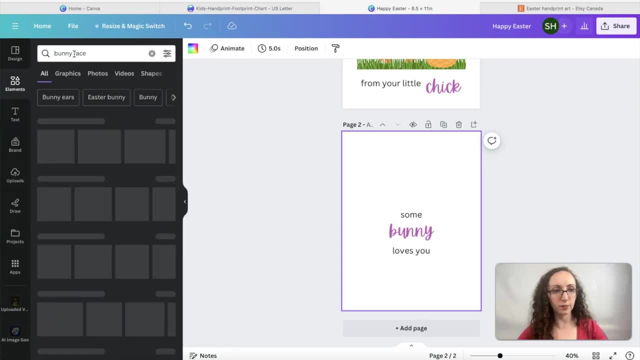 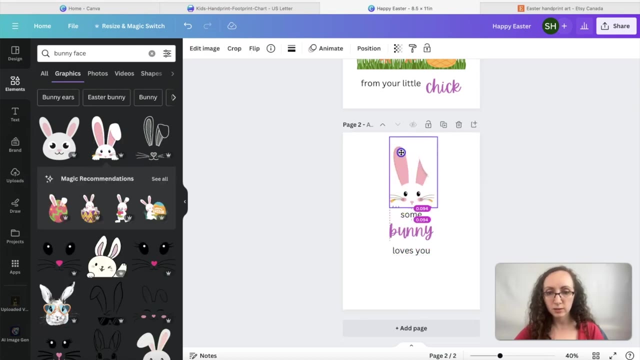 But I just wanted to get it written for now. So now we're going to go try to find Some bunny ears or a bunny face, Maybe All right. So maybe we can use something like this: Are those colors editable? I don't think so. 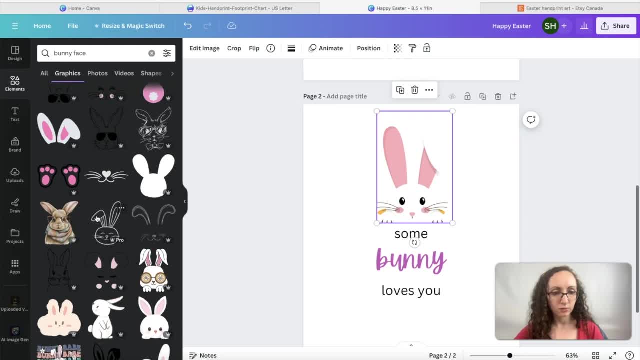 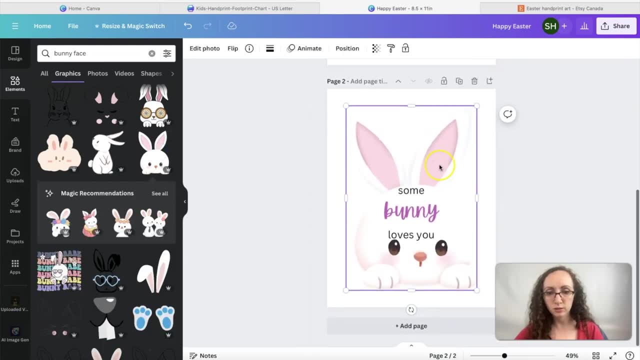 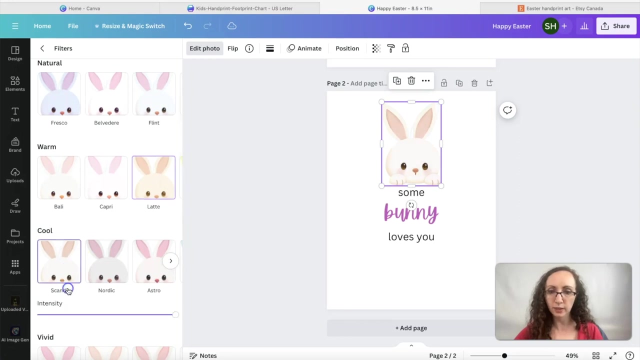 So Which other one can we use? This one's pretty cute. Okay, I'm going to go here. Maybe I'll go under edit photo See if I can get the colors. Oh, there you go. You could do something like that. 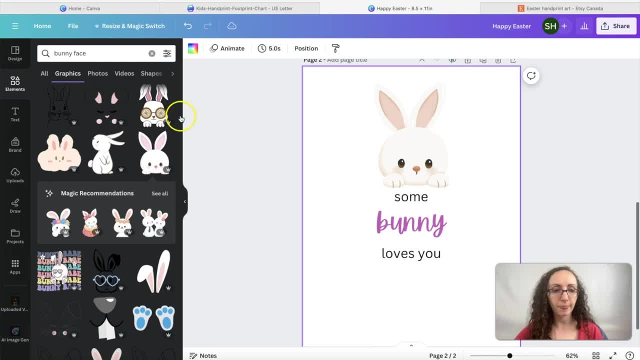 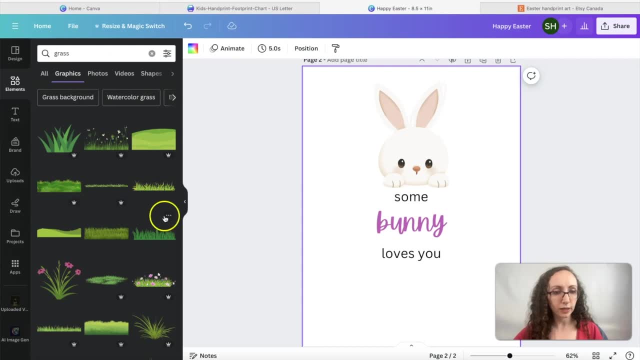 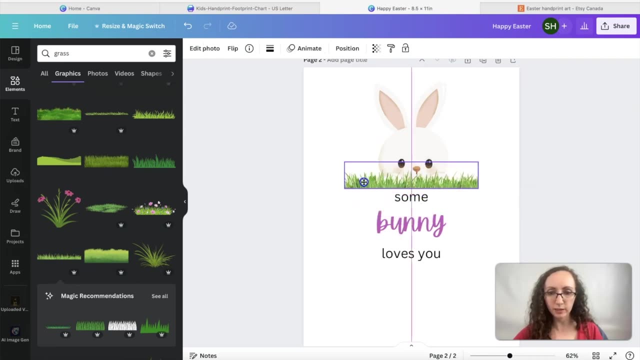 That way, it stands out more, instead of being washed out. I would maybe go find some grass again. Right, This grass. Okay, This one's a little different. We don't have to use the same one that was up there, So we're going to do this. 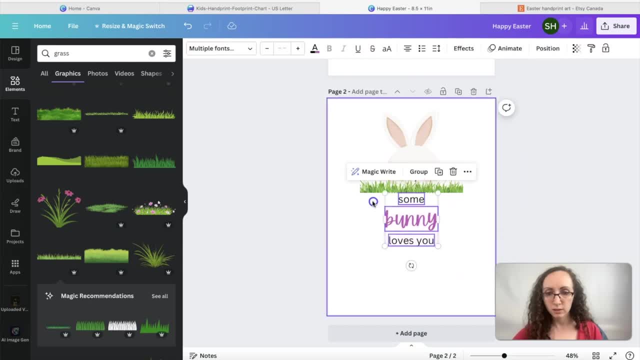 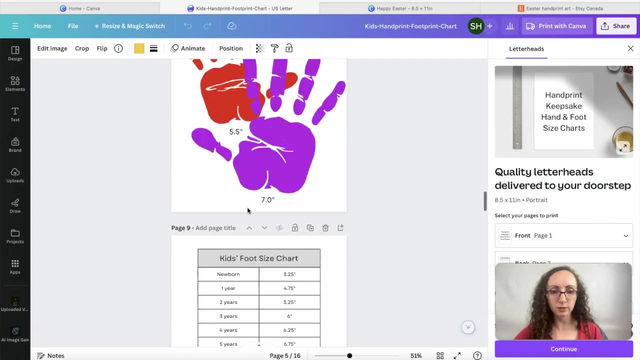 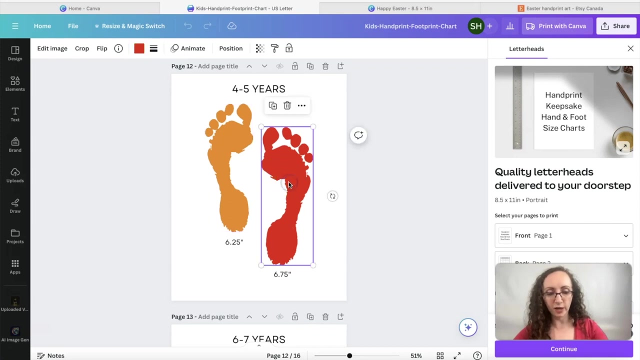 And then We're going to want to add our footprints. So I'm going to go into this sizing chart And I'm going to grab feet from maybe a five-year-old For footprint art. It tends to look a little weird. 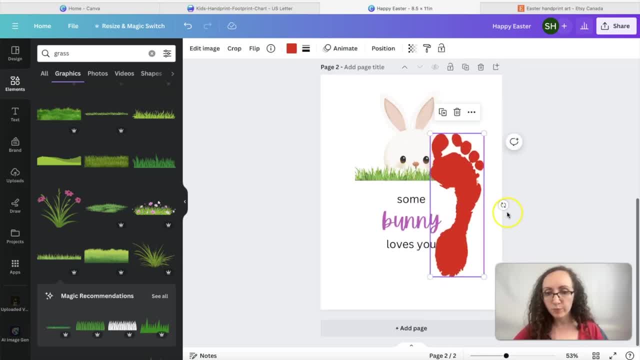 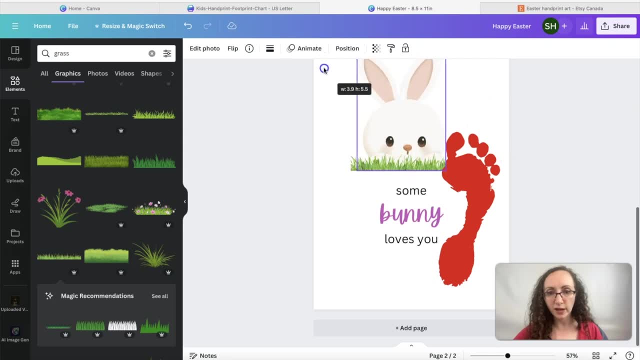 If you take feet that are Bigger than the foot of a five-year-old, In fact, even sometimes, Five is a little much Here. I'm just going to move this a little bit. So I'm going to move this text. 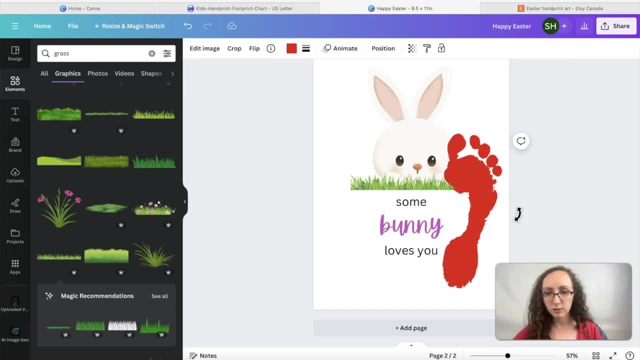 This. we're going to make room for these feet. Maybe change the size of the text a little bit So that we can move the feet closer, Something like that, And then I will duplicate it. Click this flip button And choose flip horizontal. 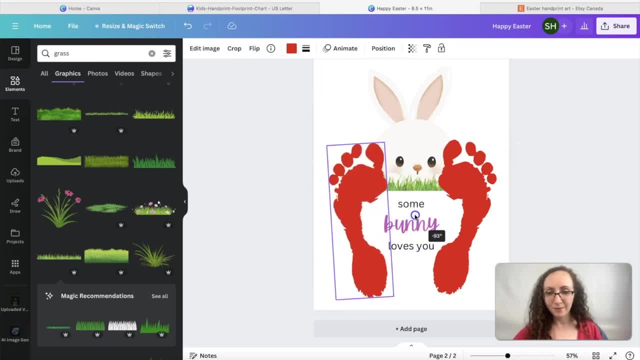 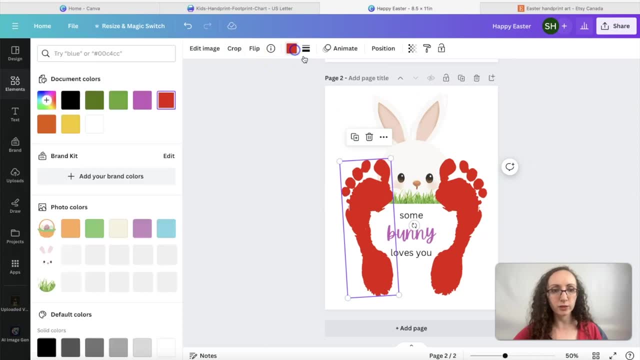 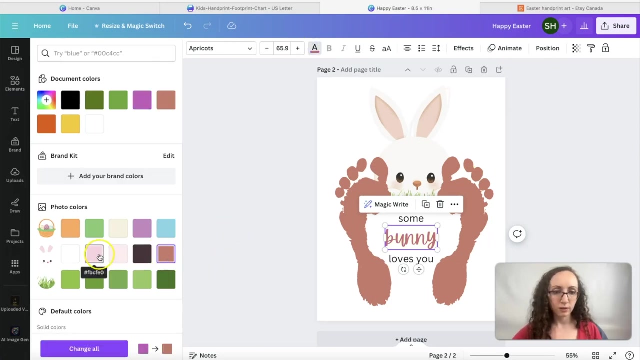 Oh, that's odd. Flip vertical for some reason. All right, Move it here, And then I will change the color For something that matches better. Yeah, So we could choose this color. All right, And then maybe we can change the color of this text here. 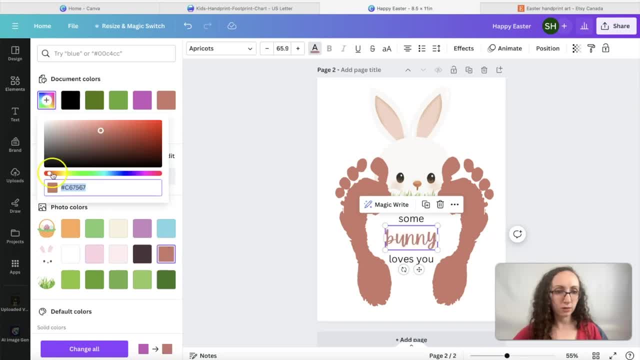 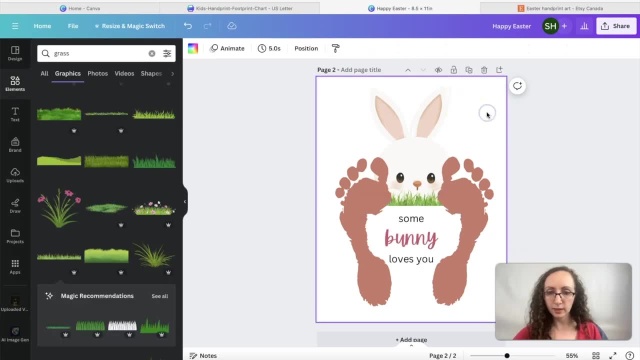 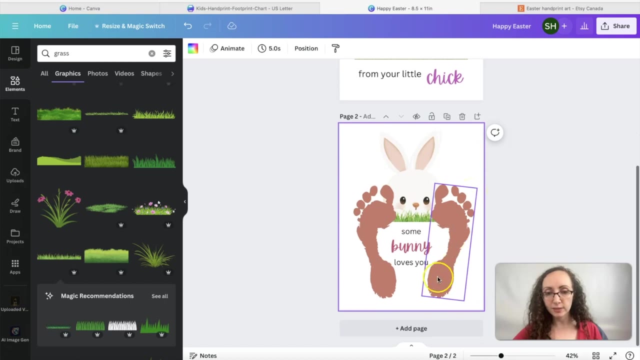 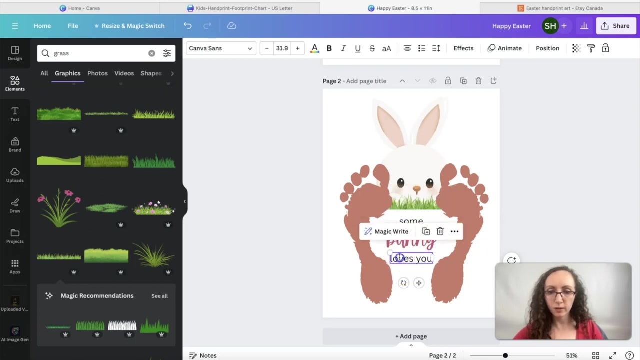 Make it something a little pinker. There you go, So something like This. So now we have this happy Easter from your little chick And we have this Some bunny loves you. The text a little bit, There you go, Perfect. 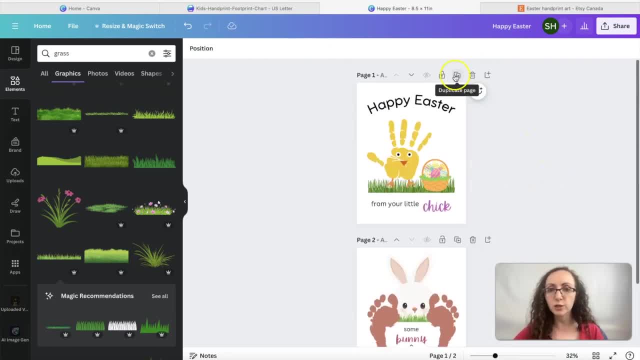 So the way that you would package this to sell it to customers Is you would go duplicate each page And you would delete the footprints and handprints On one of the pages. Oops, No, Not the text, Just the handprints. 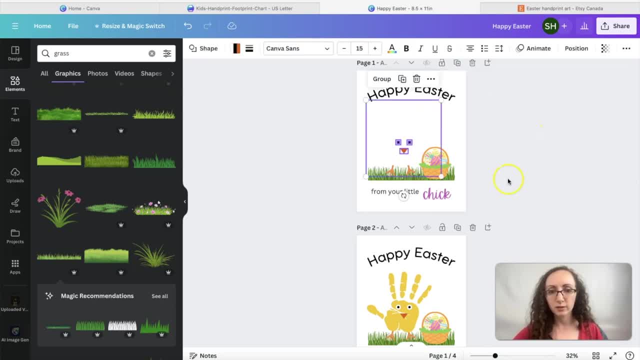 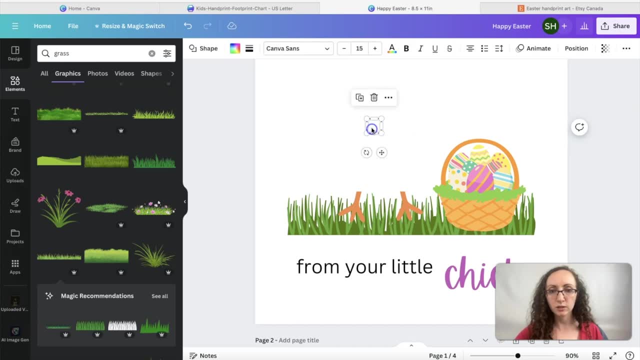 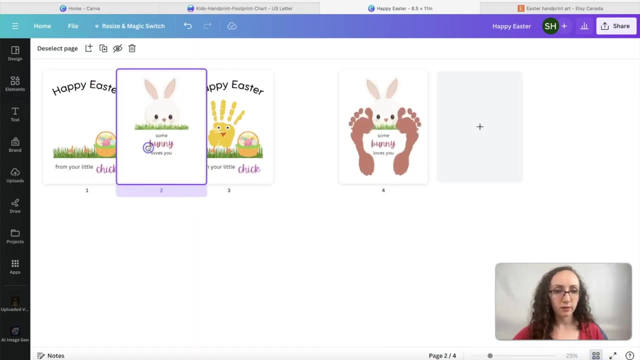 And anything that your customers are supposed to add on top. So The eyes, The beak, And there you go. So what you would be sending to your customers Is this, right here, This template that has the feet of the chick. 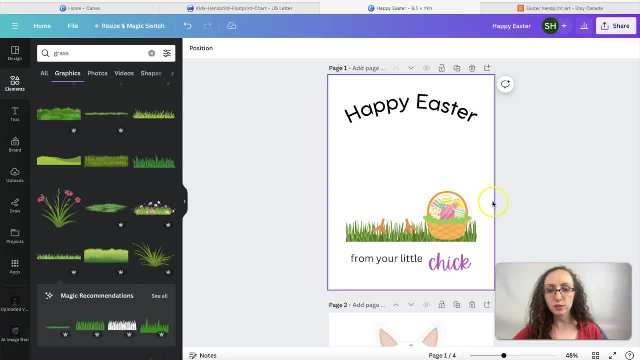 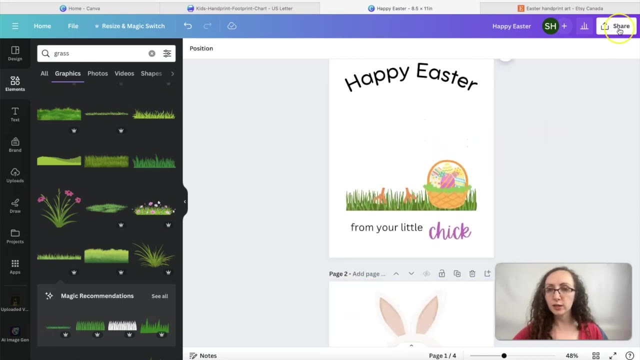 But not the chick itself, The grass, The little Easter basket with the eggs And the text, And then your customers, when they print this out, They can add their child's handprint Or footprint. So The version that I am sending to my customers. 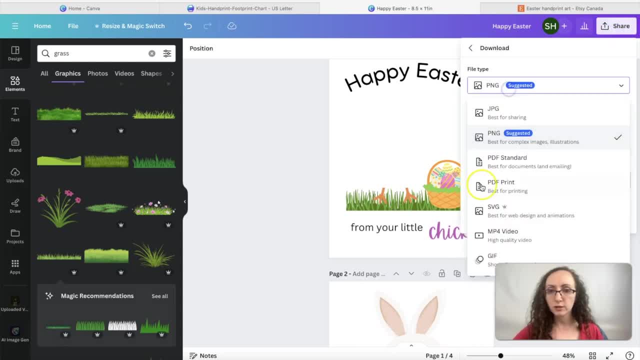 I would go here, Click, share, Download PDF, Print, Flatten PDF. This is important to comply with the graphic terms of uses So that your customers can't extract them, And then I would choose only the pages that don't have the handprints and footprints. 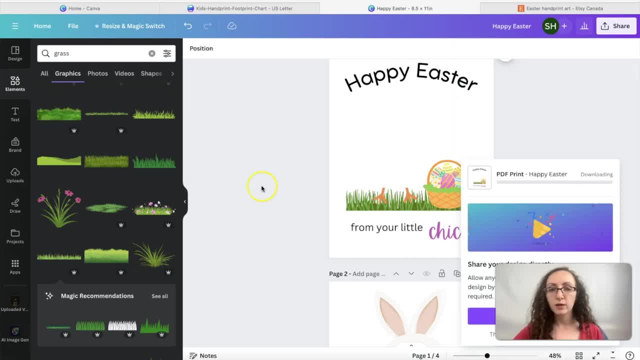 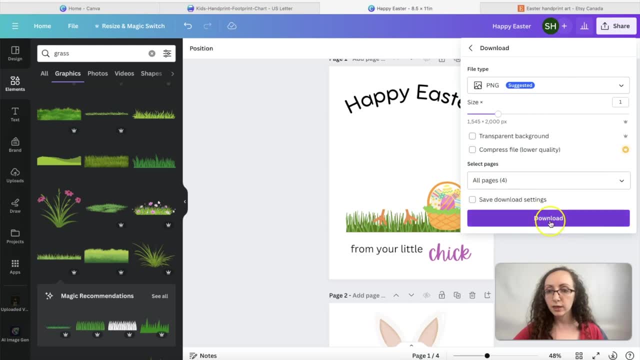 And I would download this As a PDF To make the preview images. I would go under share, Click download PNG And then download everything And then I would go create a preview image. So the way that I would do that. 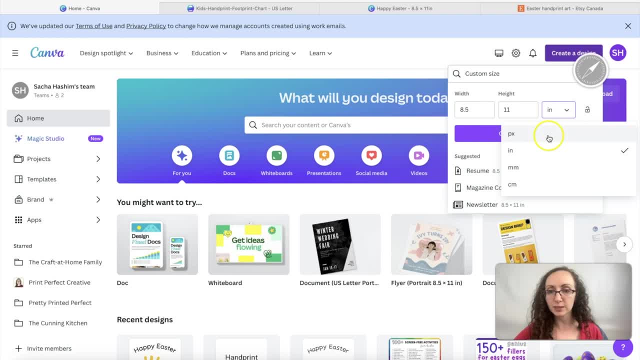 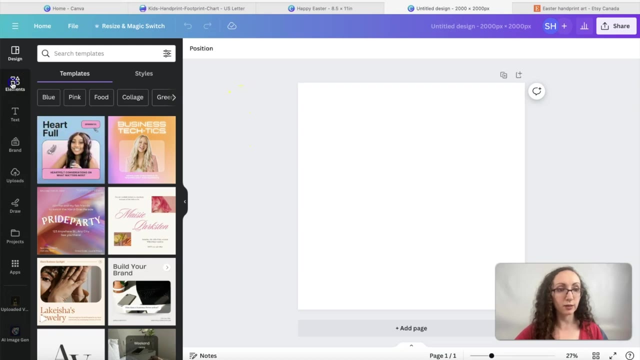 Is. I would go Home And then for If you're listing it on Etsy, You're going to want your preview images To be 2000 pixels by 2000 pixels. Create a new design And Something fun that you can do here. 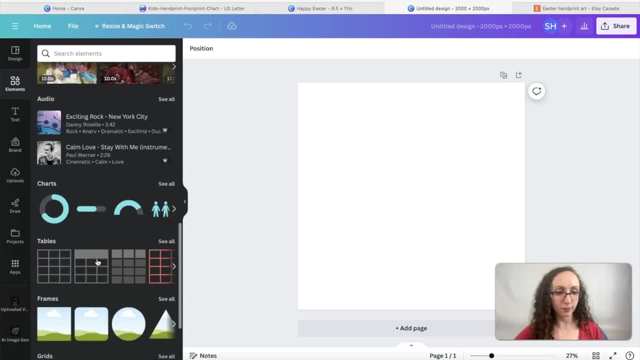 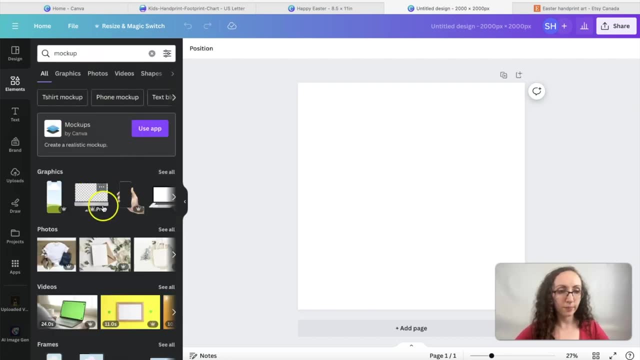 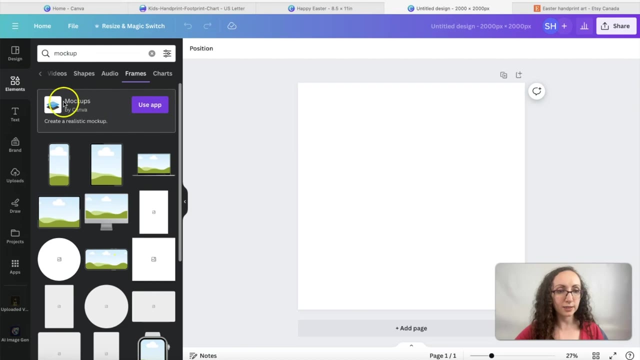 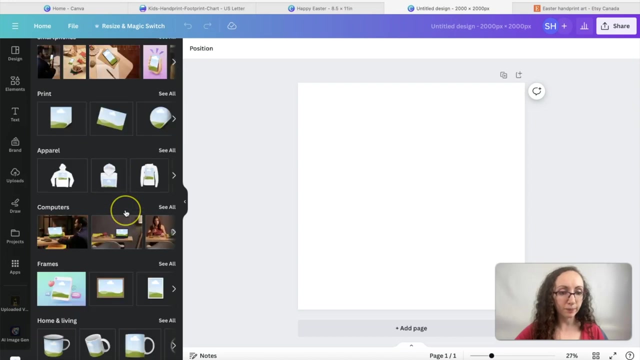 Is Create a mockup. So if I look, If I type in mockup, Okay, they have these frames here, And then you have this use app function. So if we create use app Now we can go find a frame. So if we go under frames, 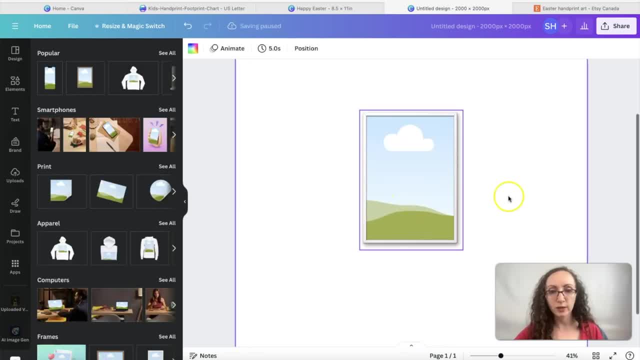 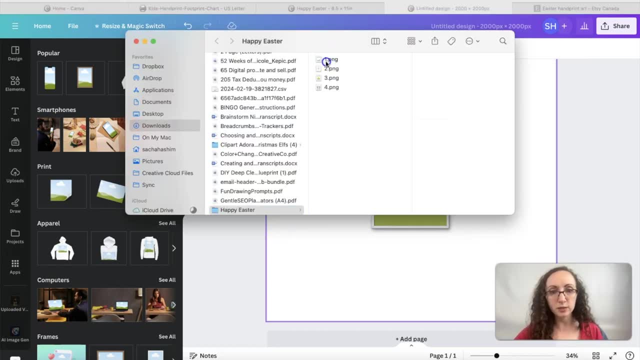 Let's see if one of them looks like a picture frame. There you go, So you would have to find one That is the right size. But if I go under Happy Easter and I download the ones That have, You would probably want to rename this. 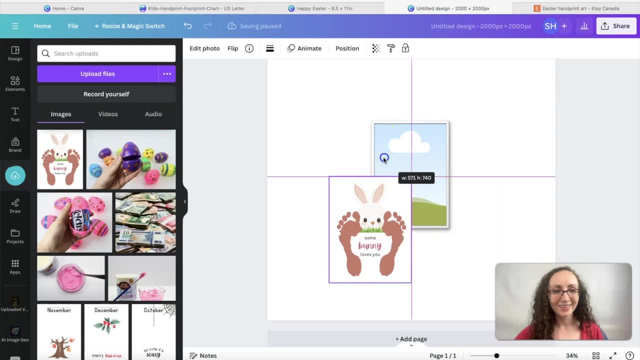 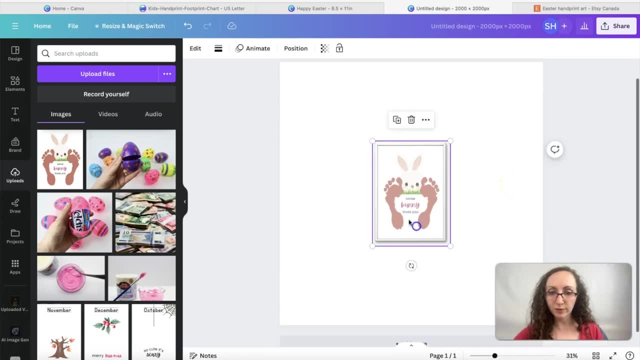 But I'm not going to waste your time By doing that now And then, If you drag it in, There you go. It's going to create this preview image That looks like a realistic mockup, So you could go put. 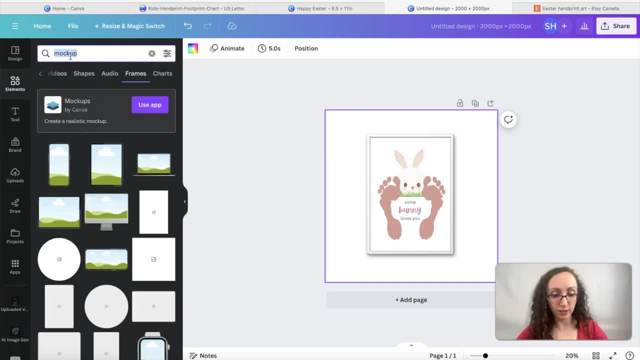 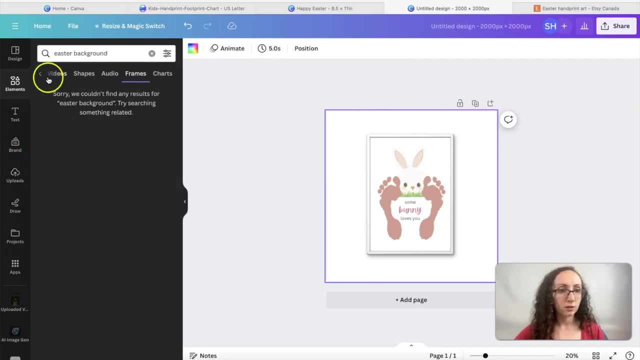 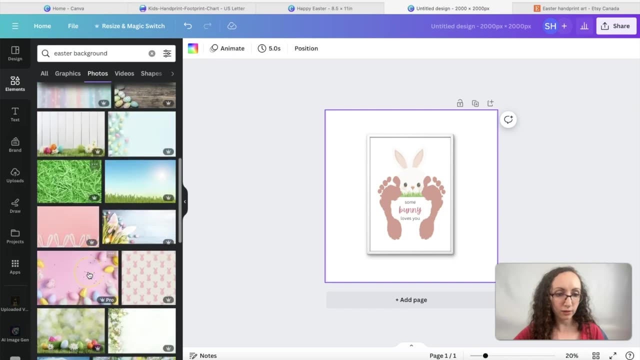 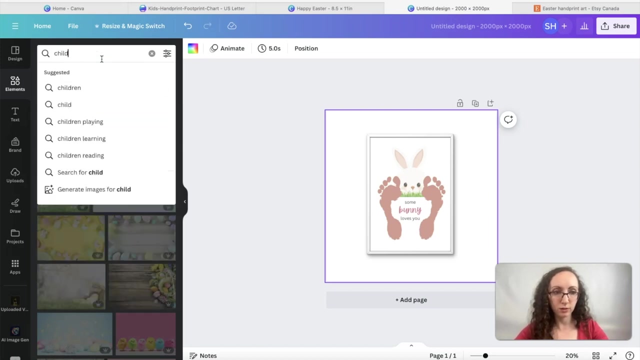 Whatever background you want, I could write- I don't know- Easter Background, Not under frames, I would do it under photos. Let's see if there's anything cute here. Maybe not, So in that case, Maybe child bedroom. 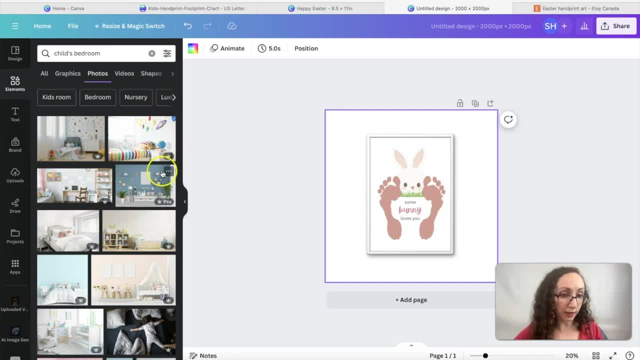 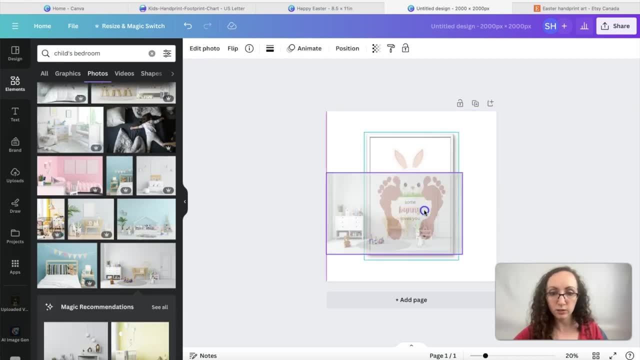 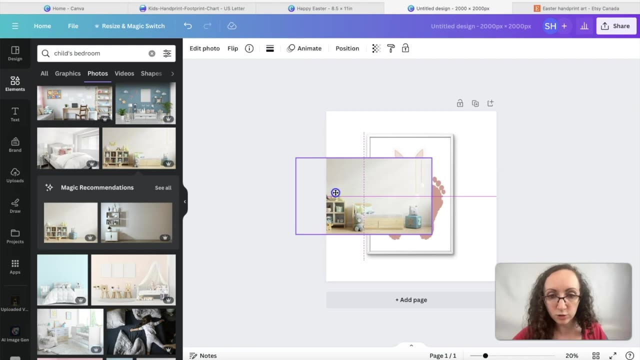 Just to give your customers a sense Of what this can look like Once they have done the handprint art And put it on their walls. I'm not a huge fan of the colors That are here. Maybe I can choose this nursery type. 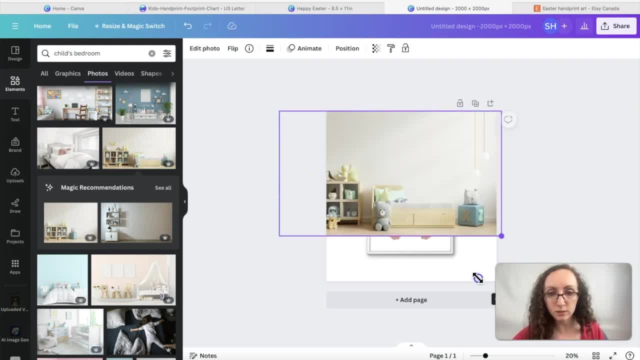 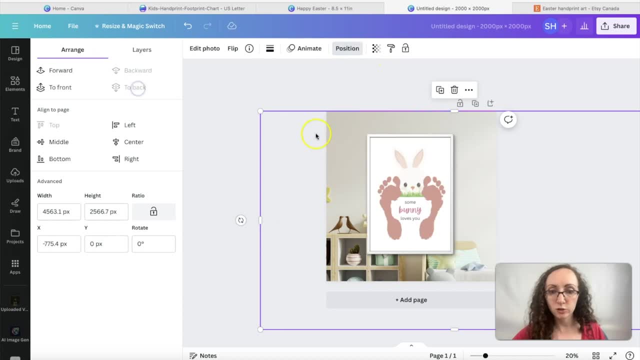 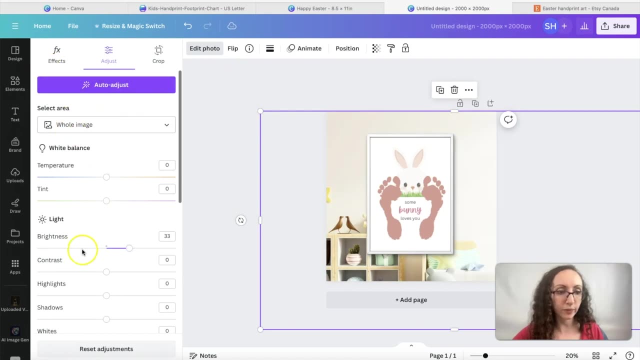 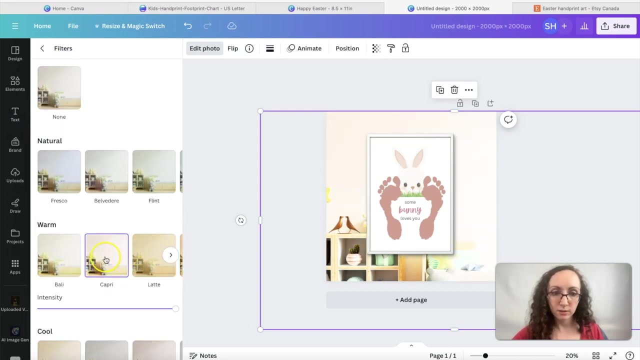 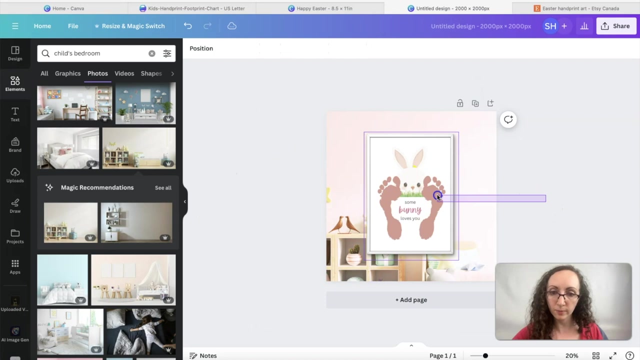 Image And Something like this Position to back. I would maybe edit this photo A little bit. The brightness, The colors- Um, Maybe I go under effects. This whimsical one is cute. It goes well with the color scheme. 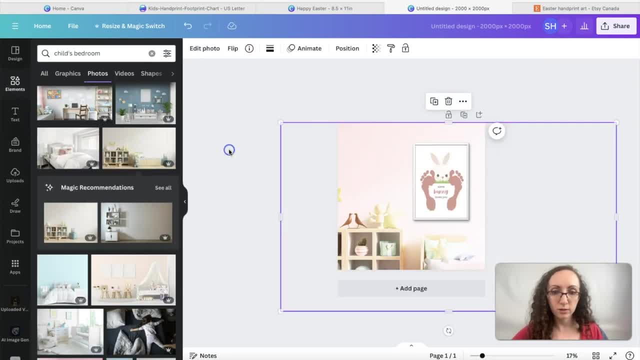 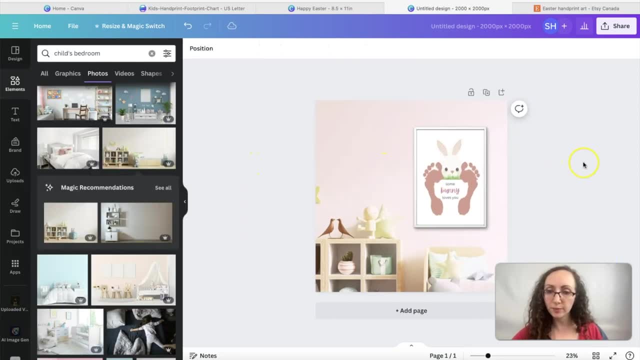 There you go. Maybe I'll go bring this brightness Back down a notch. There you go, So you could do a mockup That looks like this: Um, And then, In a subsequent page, I like to include Um. 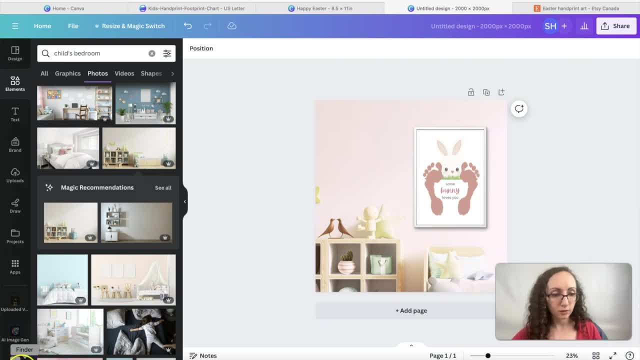 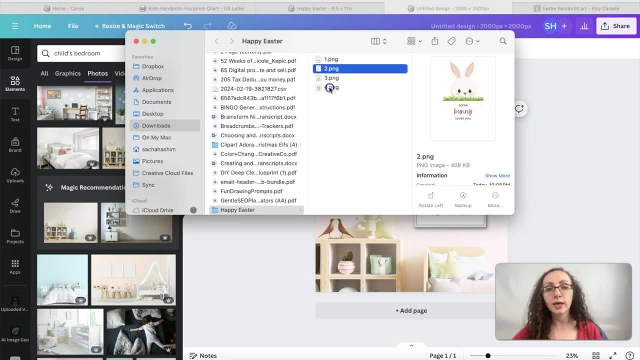 Where is it? Yeah, I like to include Both The image Without The handprints Or footprints And the image With The handprints Or footprints, Just to give Your customer an idea Of what they're going to receive.